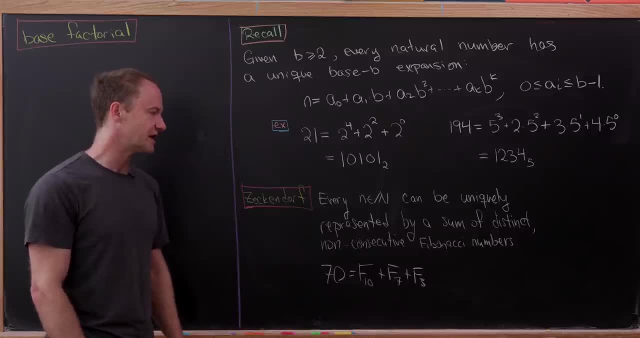 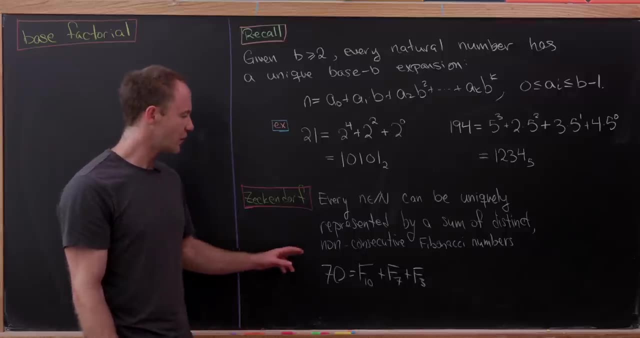 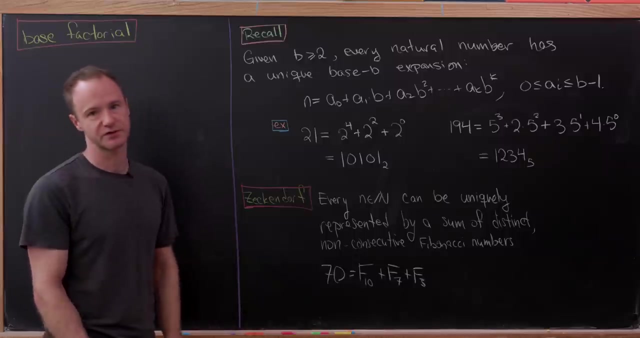 psyched. So it says that every natural number can be uniquely represented by a sum of distinct, non-consecutive Fibonacci numbers. So if you don't add this rule that you have non-consecutive Fibonacci numbers, then you do not get a unique representation. You can play around with this. 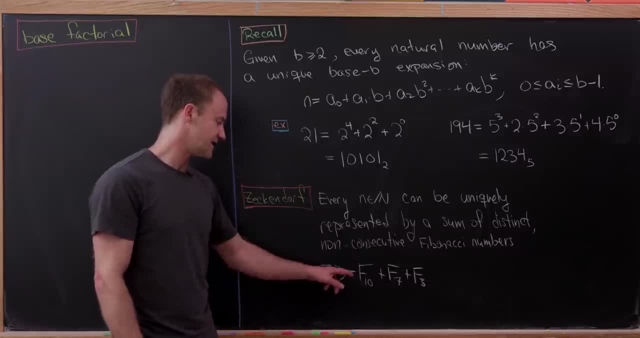 if you'd like to. So let's notice that 70 can be written as the 10th Fibonacci number plus 3 times 5 squared. plus 2 times 5 squared. plus 3 times 5 squared. plus 3 times 5 squared. 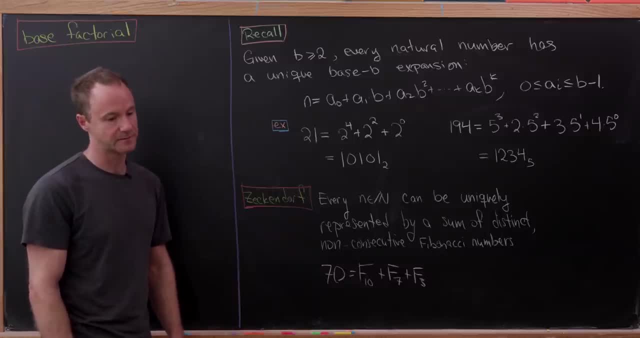 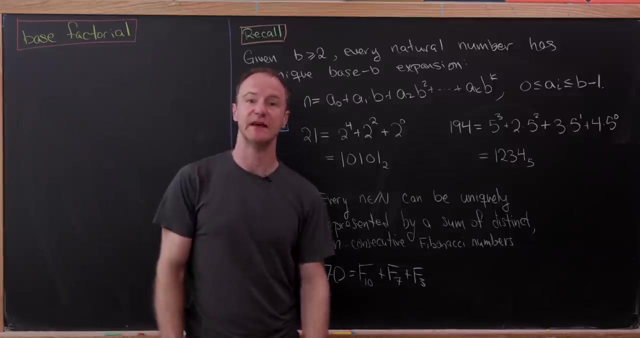 plus the 7th Fibonacci number plus the 3rd Fibonacci number And, just as a heads up, 55 plus 13 plus 2.. Okay, so, now that we've kind of recalled all of this kind of background information, let's talk about our real idea here, which is base, factorial. Okay, so let's start by 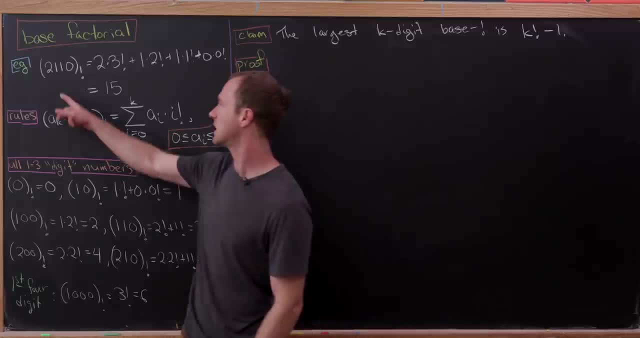 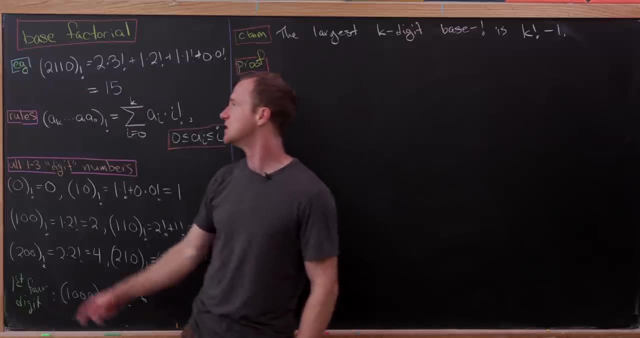 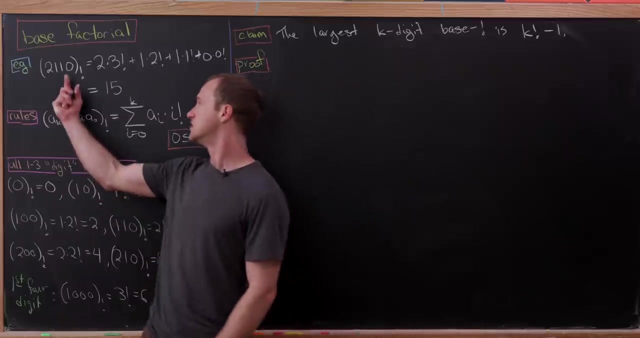 dipping our toes into this factorial number system by looking at the number 2110, base factorial, and that's the notation we'll use. So the place value here is the multiple of- well, whatever factorial you're at. So this furthest right digit is a multiple of 0 factorial. This next digit will be a multiple of 1 factorial. 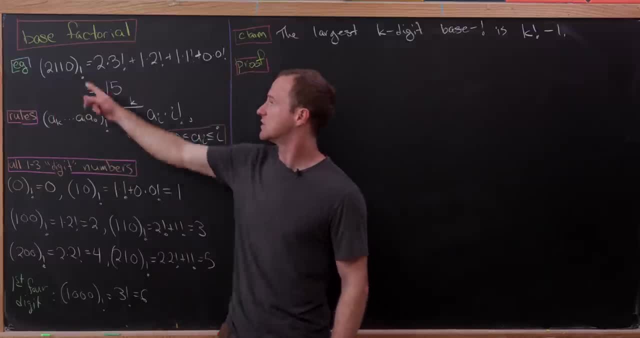 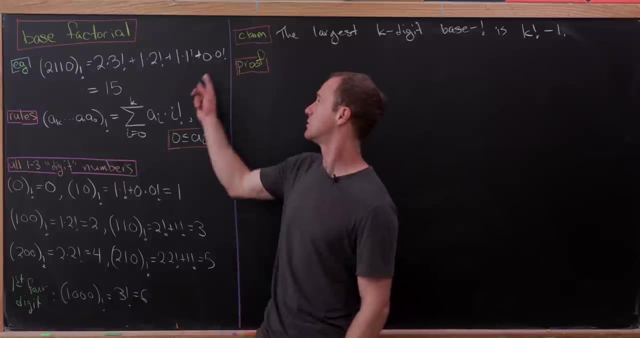 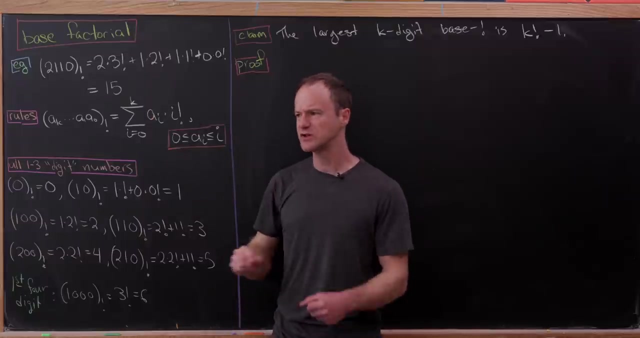 and then 2 factorial and then 3 factorial. So this number expands out to 2 times 3 factorial plus 1 times 2 factorial, plus 1 times 1 factorial, plus 0 times 0 factorial, And adding all that up you get the number 15.. And so, to put it like into a bigger package, 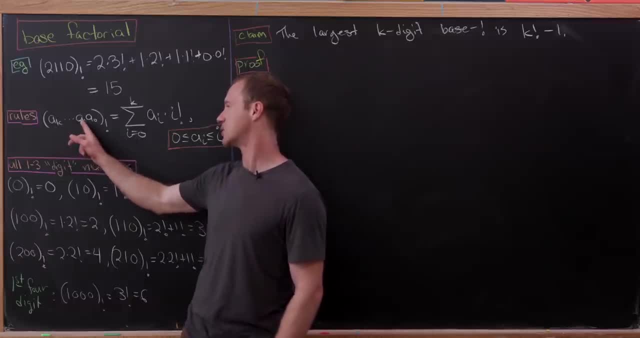 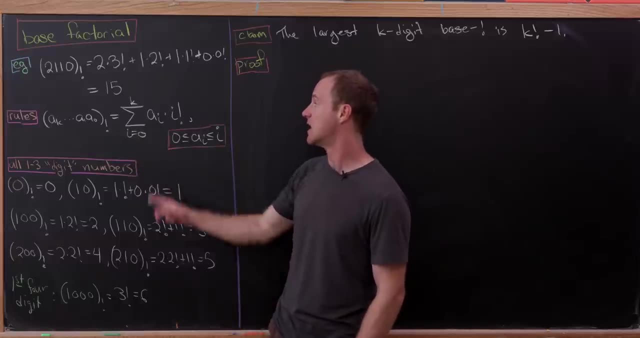 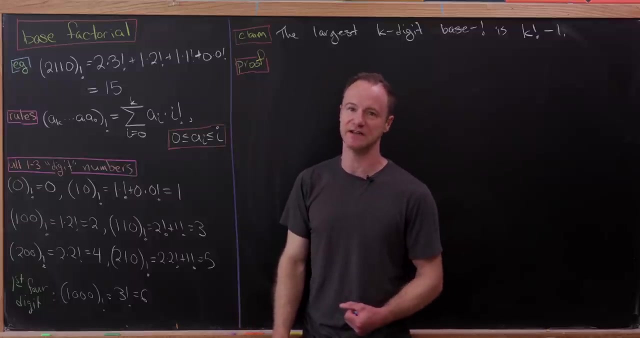 you would say that the number AK, AK minus 1 down to A1A0 factorial is the sum, as I goes from 0 to K, of AI times I factorial. And then there's got to be some sort of rule on the size of the digits. 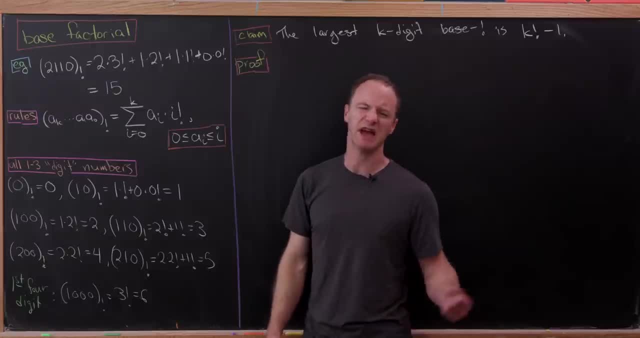 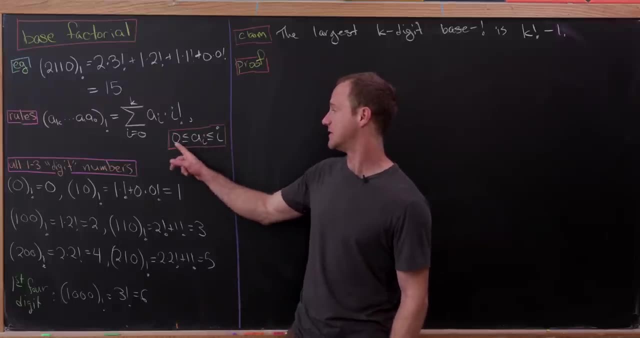 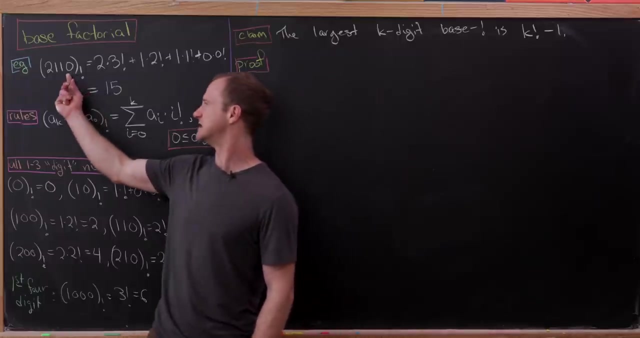 There always was, when we were talking about base B and even in the case of Fibonacci. And in fact the rule is this: We need AI to be between 0 and I, and we can include I here. Notice that means that this 0 factorial digit is always 0. 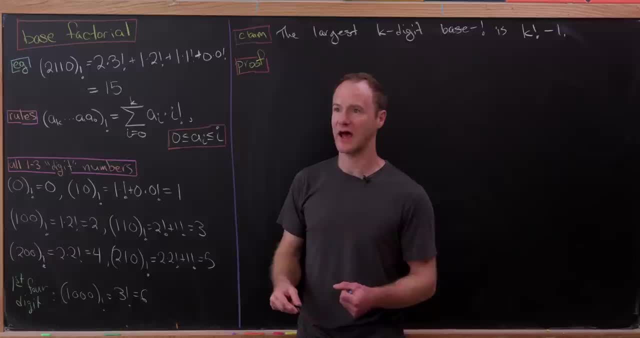 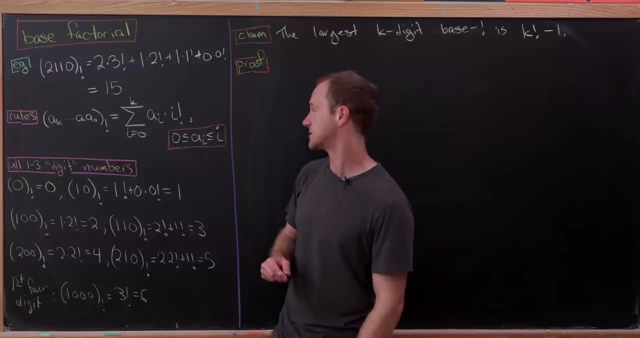 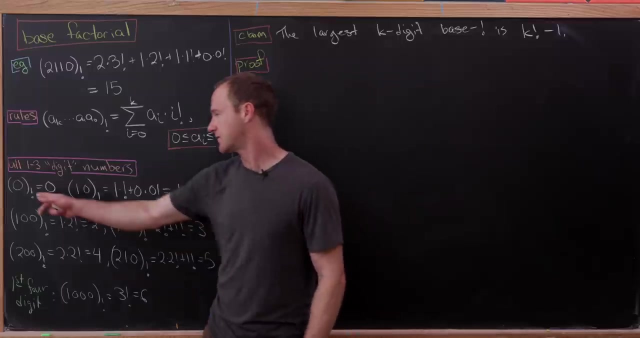 And I'm not exactly sure why we keep that one around, as it just always gives us the number 0, but in the references that I was looking at, that's always part of it. Okay, so let's look at all of the 1 to 3 digit numbers in base factorial. So the first one would simply be 0. So I don't think there's. 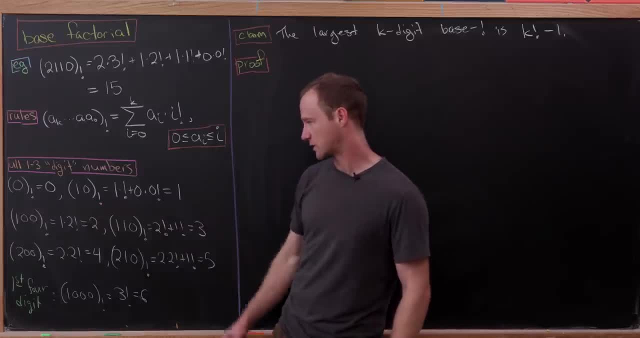 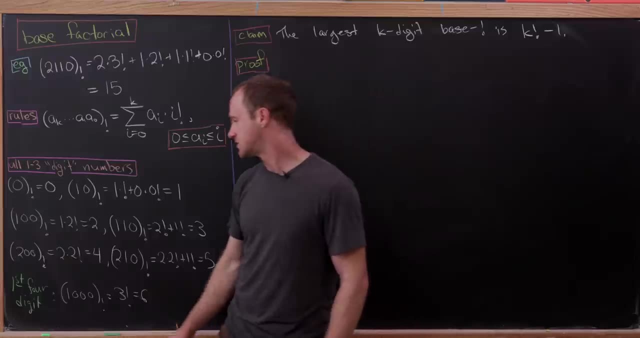 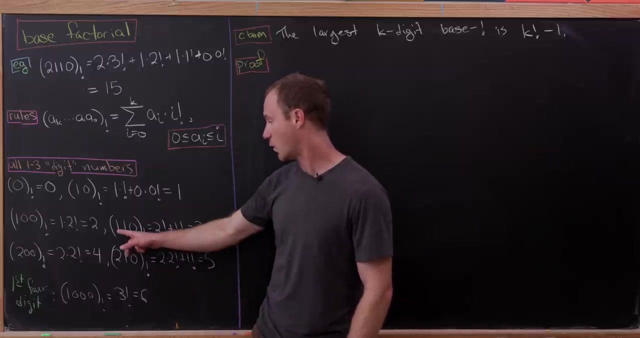 much to say there. Then you've got 1, 0 base factorial. So that's going to be 1 factorial plus 0 times 0 factorial, In other words the number 1.. And so the number 2 is 1, 0, 0 factorial. And then the number 3 is 1, 1, 0 base factorial. 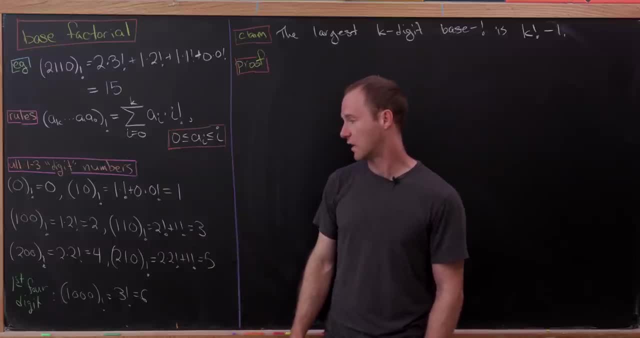 That's because that's 2 factorial plus 1 factorial And then, as you can see, you can easily represent the number 4 and the number 5.. And that's all we have. Notice that this number is most definitely the largest as the 2 factorial place. 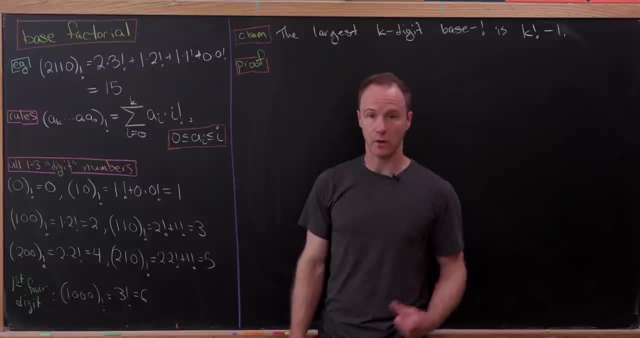 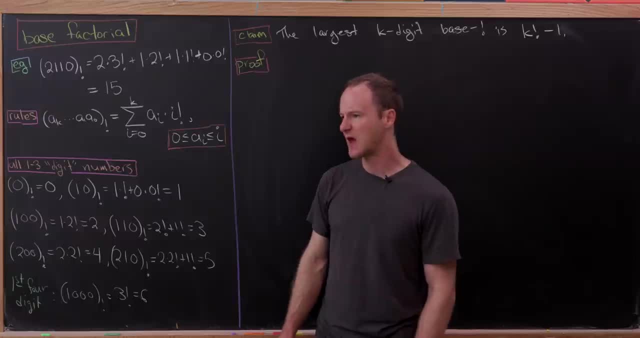 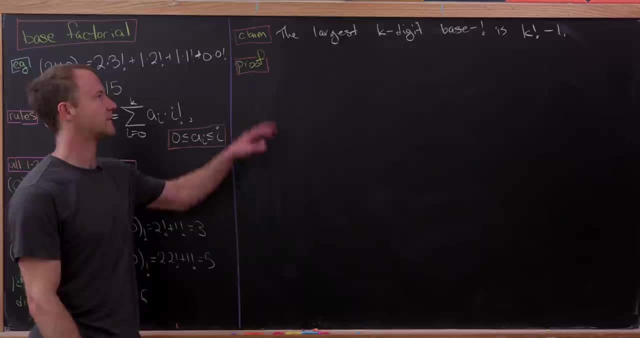 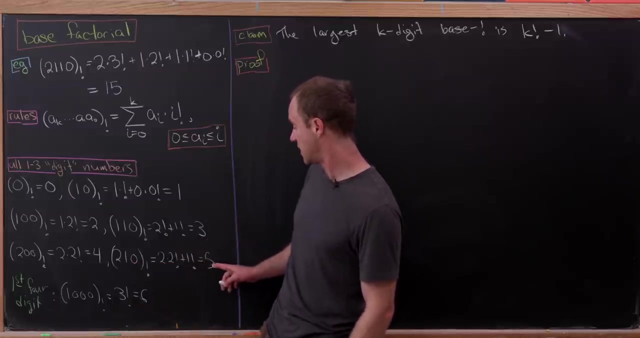 sub factorial is 6, and that's actually going to be an important little fact- or that's an example of an important little fact that we'll use later- and that is that the largest K digit base factorial number is in fact, K factorial minus 1. that's exactly what we see right here. so notice: the largest 3 digit is 3. 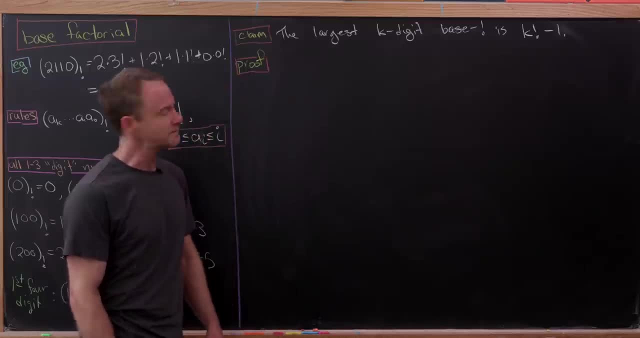 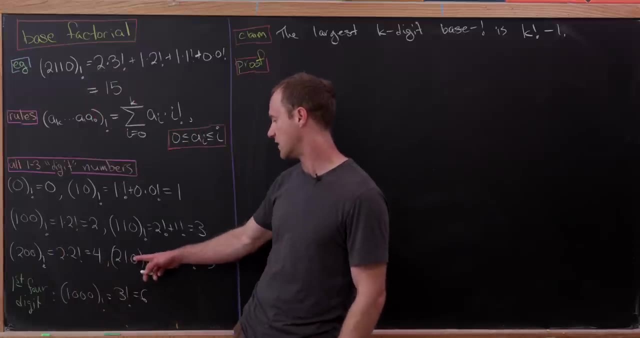 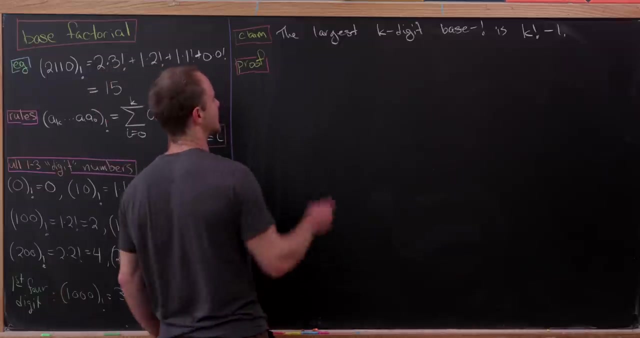 factorial minus 1, aka the number 5, and so it's pretty clear what number this is. it's just the number that achieves all of the maximum digits, so we just have to show that that actually sums up to K factorial minus 1, and it's not too bad. 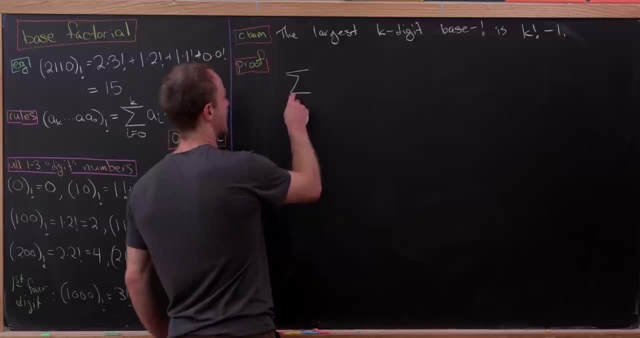 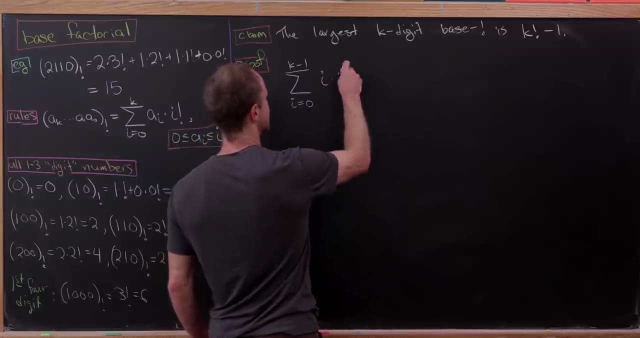 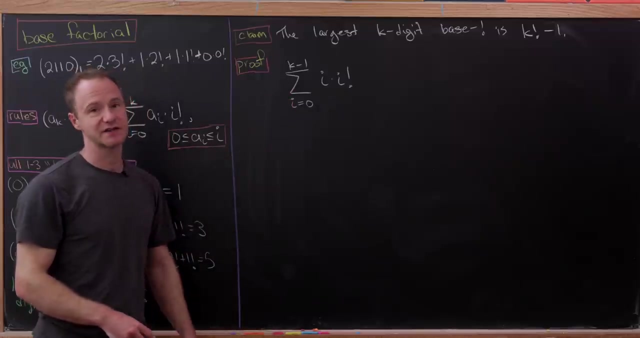 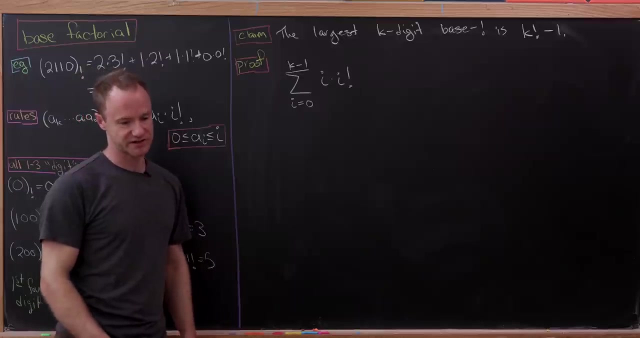 so let's look at this. we'll have the sum, as I goes from 0 to K minus 1 of I times I factorial minus 1 factorial. so again, that's achieving the maximum digit. there. notice, I stop at K minus 1 because, well, we've got a zeroth digit and so this is like K total digits. 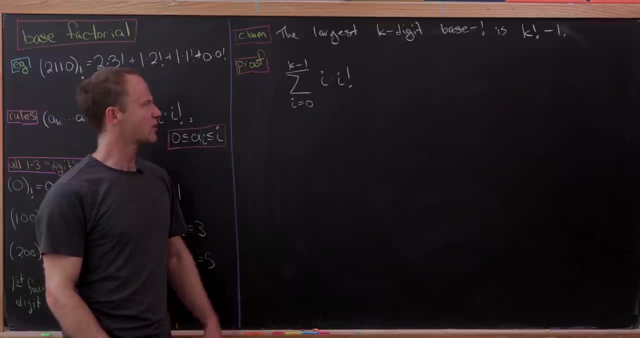 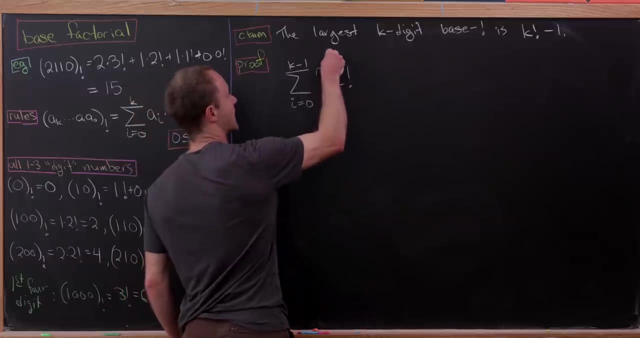 okay. so next up, we're going to take this number I and write it in kind of a fancy way. so I'll take this number I and I'll write it as I plus 1 minus 1, and then we'll distribute this I to K minus 1, and then we'll distribute this I to K minus 1. 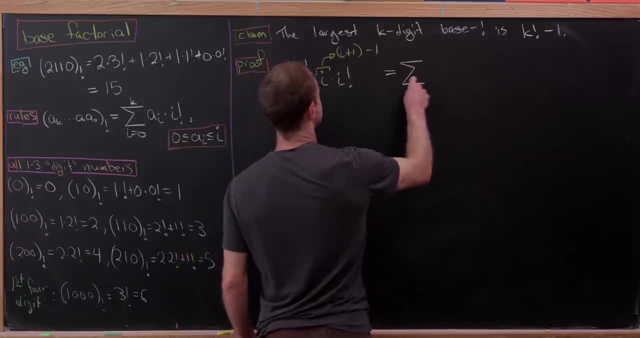 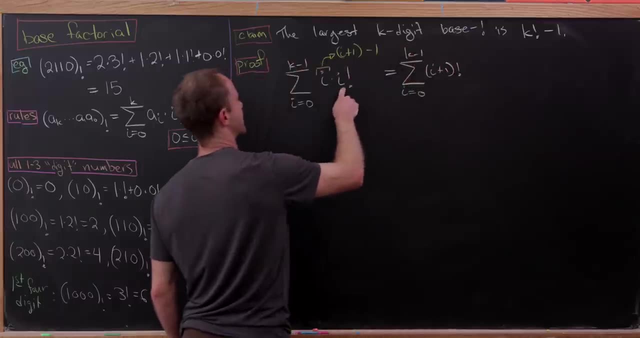 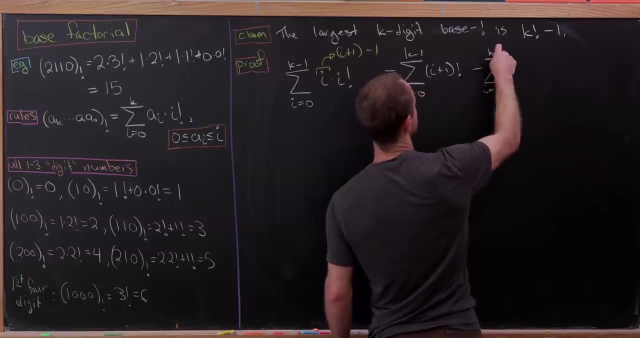 I factorial over it. so that'll leave us with the sum as I goes from 0 up to K minus 1 of I plus 1 factorial. that's what we get from I factorial times I plus 1 and then minus the sum as I goes from 0 to K minus 1 of I factorial. 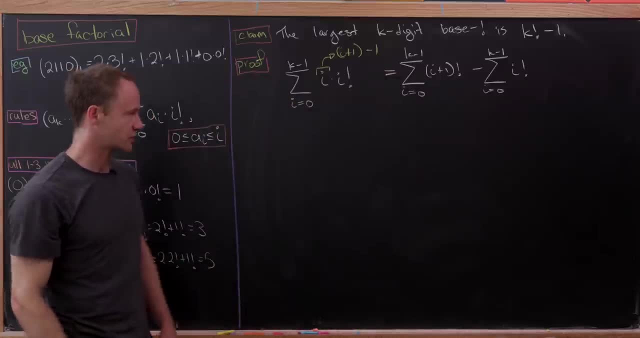 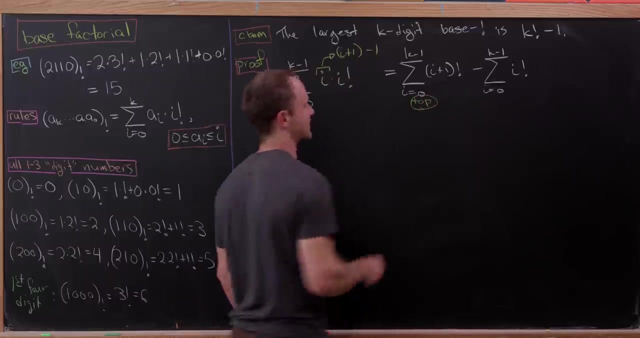 that's what we get from distributing the 1 on to the I factorial. oh, but check it out. we're essentially done at this point. notice that we could perhaps re-index this, or maybe notice that the only thing that survives after taking the difference here and doing kind of the 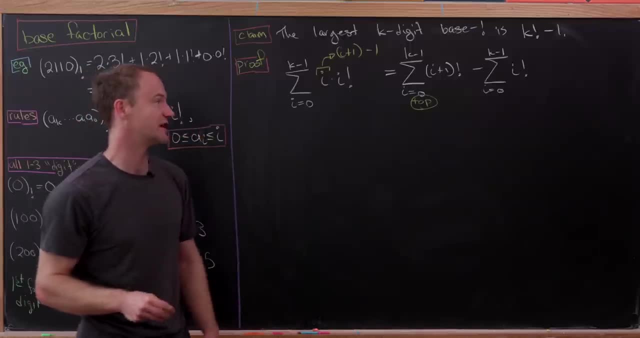 obvious. telescoping action would be the top term of this and the bottom term of this. no, we could get real fancy and re-index this, but I don't think we really need to do that. so the top term of this first sum, well, that's K minus 1. 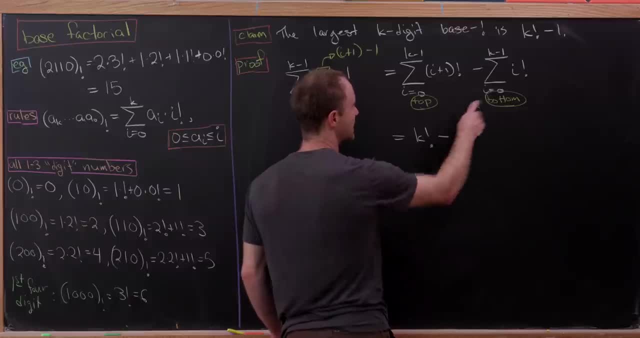 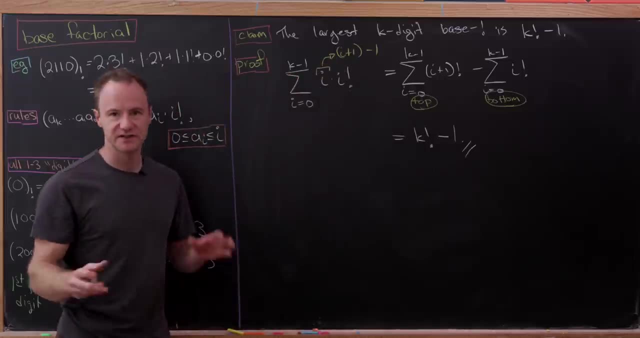 plus 1 factorial aka K factorial S term of this second sum is 0 factorial aka 1.. So there we have it. We've just done a little bit of an argument about why the largest k-digit base factorial number is k factorial minus 1.. And now, 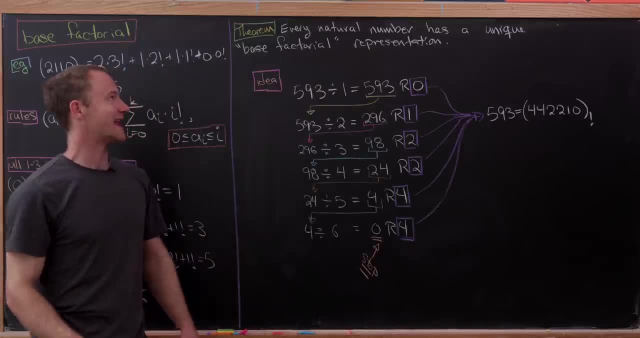 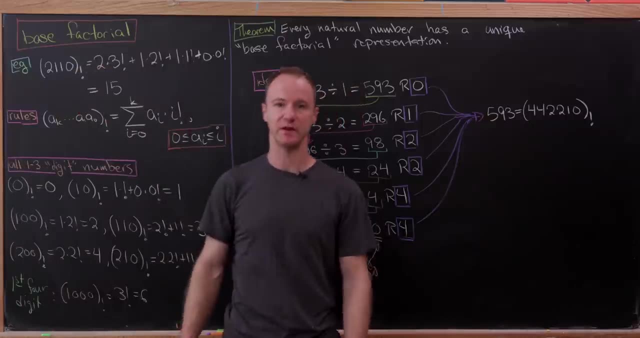 we're going to move on to our main result. So our main result is that every natural number has a unique base factorial representation, where by base factorial I mean this kind of stuff that we did over here. So this proof is constructive, and so, that being said, I've worked out this little. 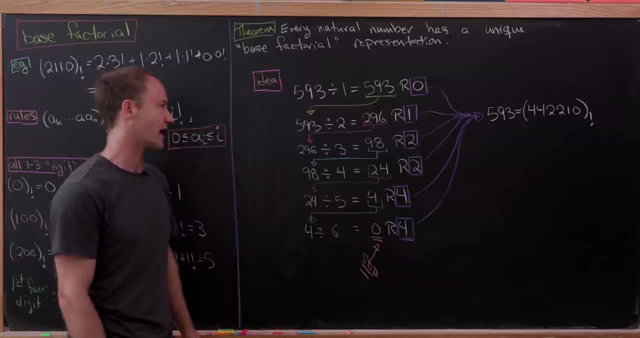 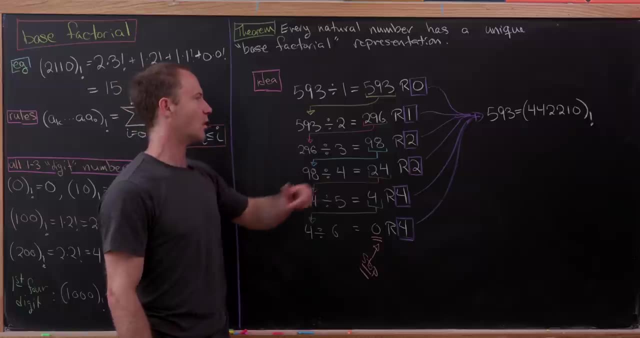 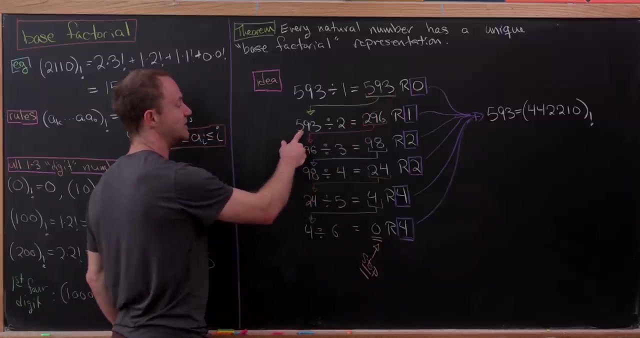 example of how it goes before we jump into the generality. So I've taken the number 593 and the first thing that you do is divide it by 1, take the quotient and the remainder, And then this quotient will become the new dividend. So in this case, 593 is still 593.. Then you're going to 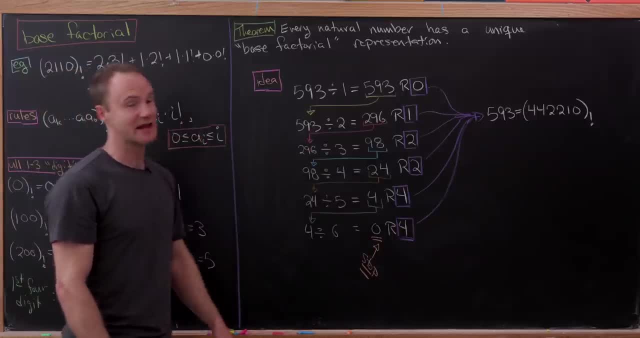 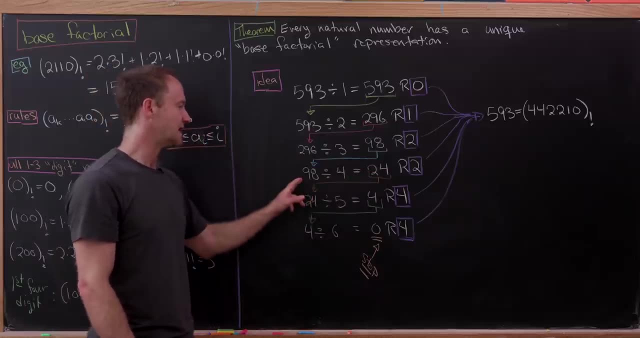 divide it by 2.. keep the quotient and save the remainder for later, and then keep going. So you'll take 296 divided by three quotient remainder, 98 divided by four quotient remainder, and then 24 divided by five quotient remainder. 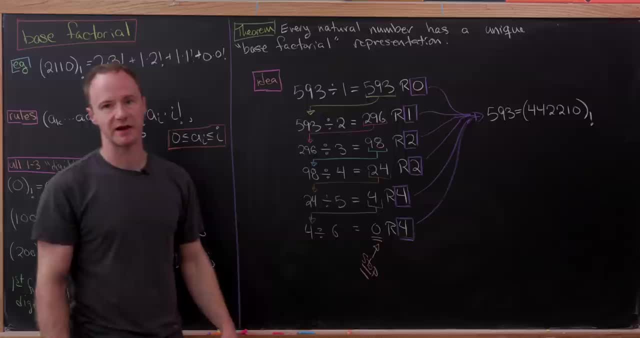 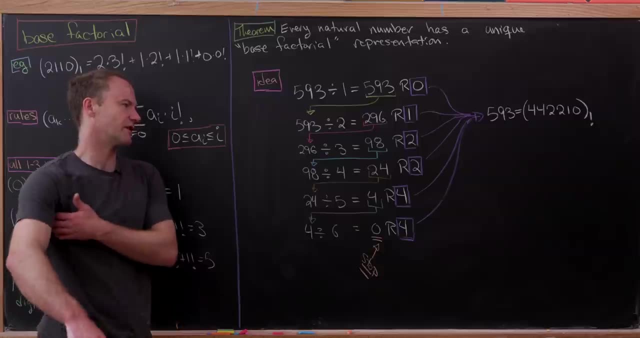 and then finally four divided by six, quotient remainder, And at some point you'll get a quotient of zero, and that's when you know to stop. And so this looks a lot like the Euclidean algorithm, except instead of taking the remainders, 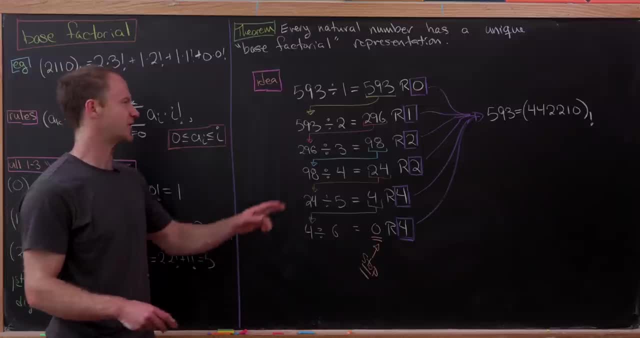 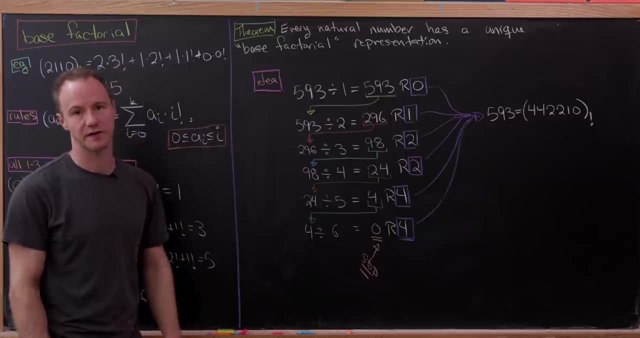 and turning them into your new quotients, you're doing something a little bit different. You're continually increasing what you're dividing by by one, And so I think this is a pretty interesting algorithm. Okay, and then you're gonna take the remainders. 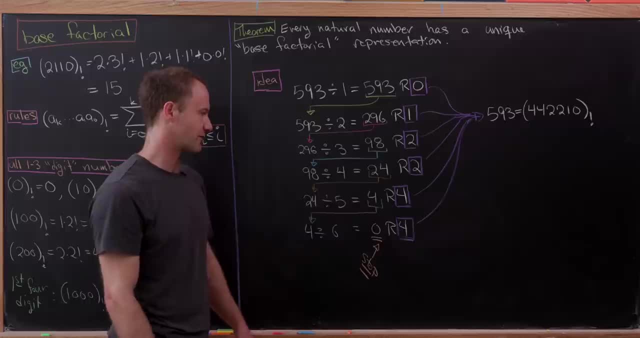 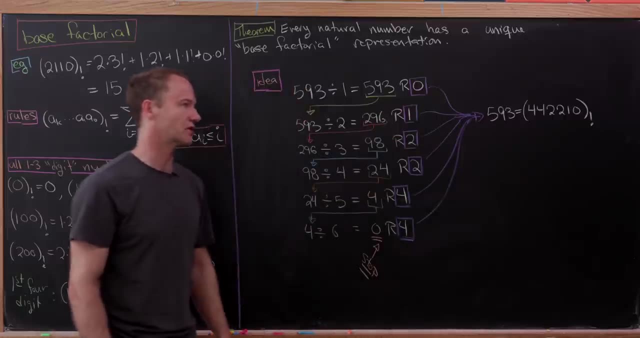 starting with the last one, and form your factorial representation. So we'll have four, four, two, two, one, zero base factorial is your original number. Okay, so now let's jump into the general proof of why this works. 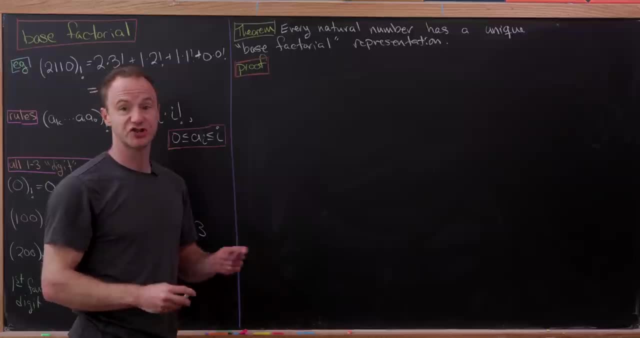 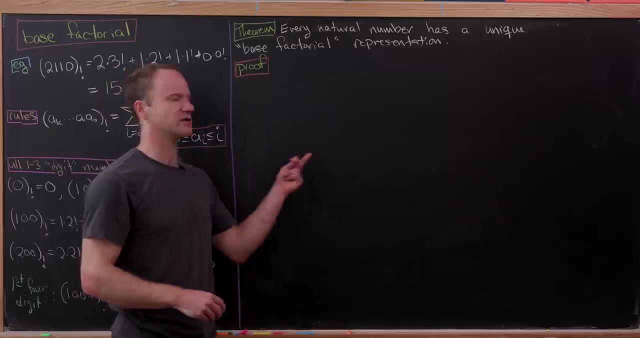 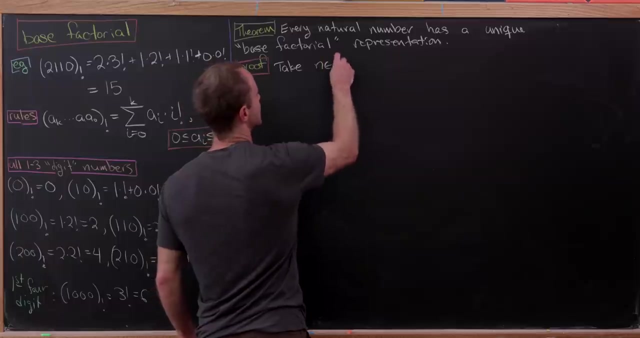 and why it gives us a unique representation. So our general argument will rely on building two sequences, And those sequences will be like the remainders and the quotients that we saw during our example. Okay, so let's take some arbitrary natural number n. 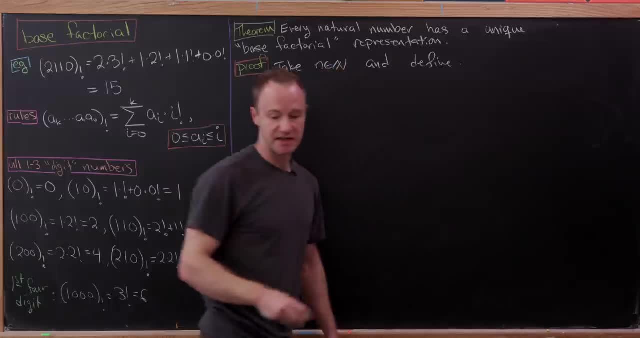 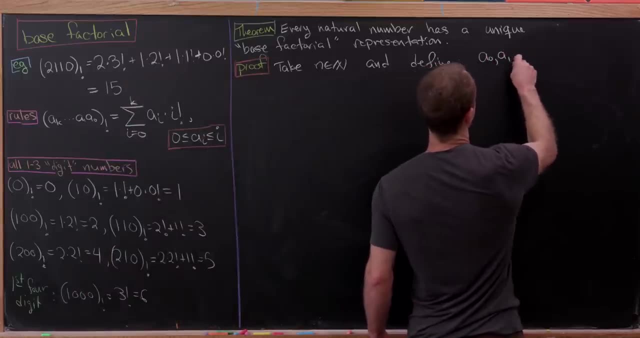 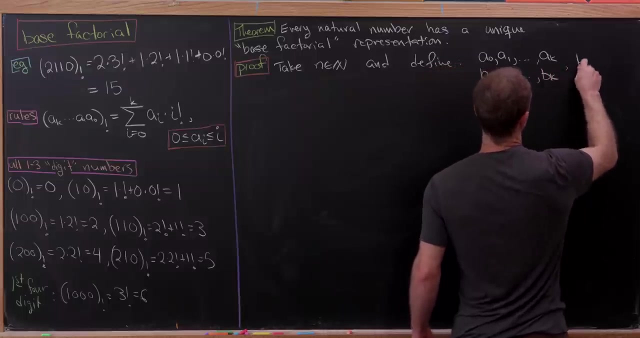 and then define the following sequences. So I'll call them like a sub something and b sub something. So we'll have a zero, a one up to a k, and likewise b zero, b one up to b k. And we're gonna define those by the following rules. 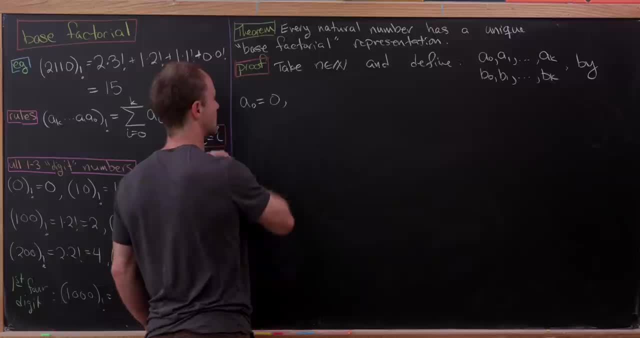 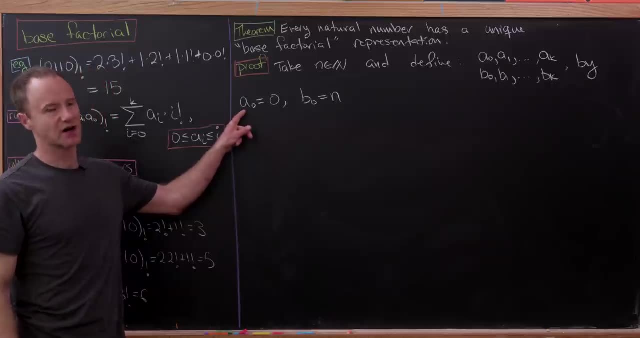 And so you'll start with a zero equal to zero, and then b zero equal to n. That's like your first digit, which, as we talked about before, is always zero, And then this n. well, that's the first thing, right. 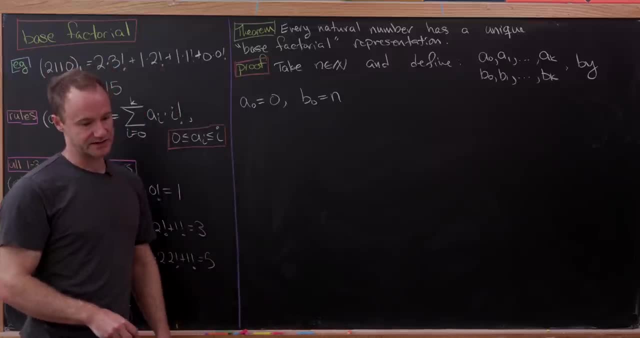 And then this n? well, that's the first thing right. And then this n well, that's the first thing right, As we saw in our example. Okay, and then you're just gonna repeatedly do like some division. 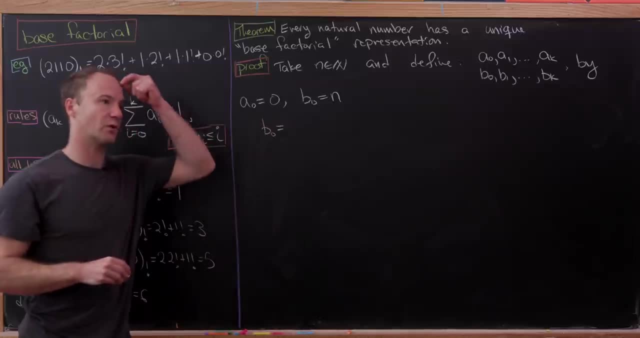 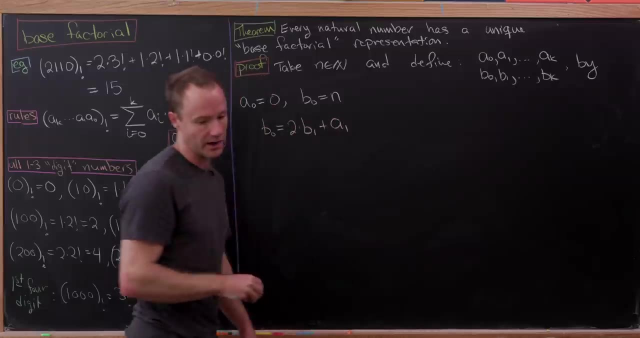 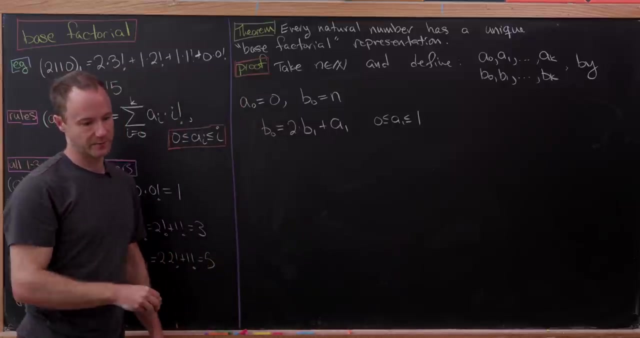 So let's take b zero and do the division algorithm where we divide by two. So this'll be equal to two times b one plus a one, And here a one will be between zero and one, again by the division algorithm. And now we're gonna continue. 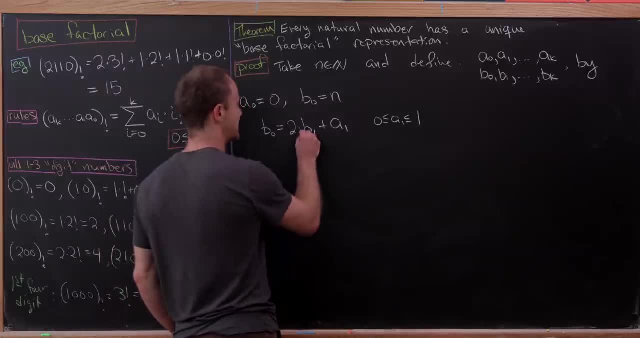 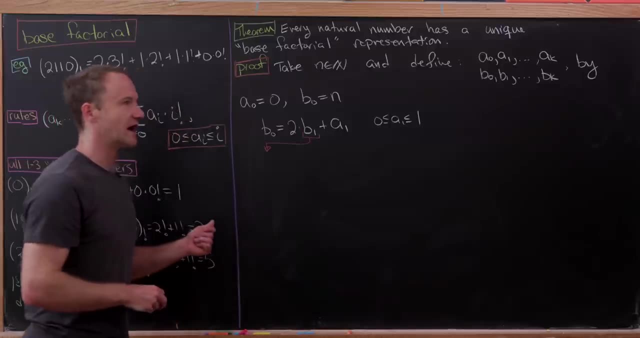 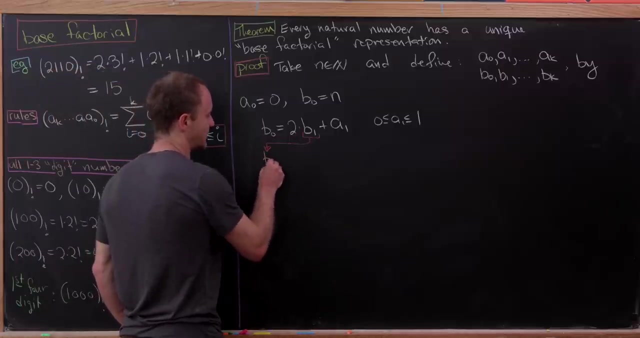 to play this game. so we'll take this b1 and move it down here. it'll be the new thing that we're dividing into, and then we'll define our b2 to be the quotient after dividing by 3. okay, so let's see, we'll have b1 goes down here, then we're dividing by 3. 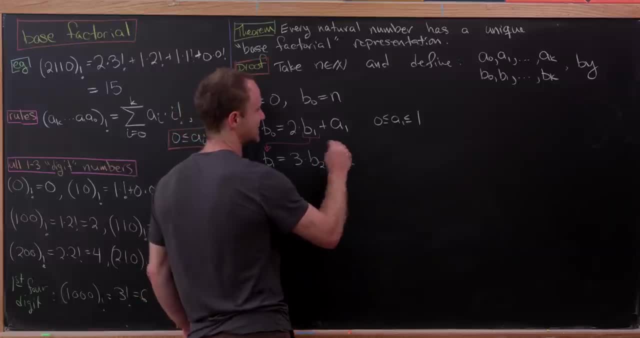 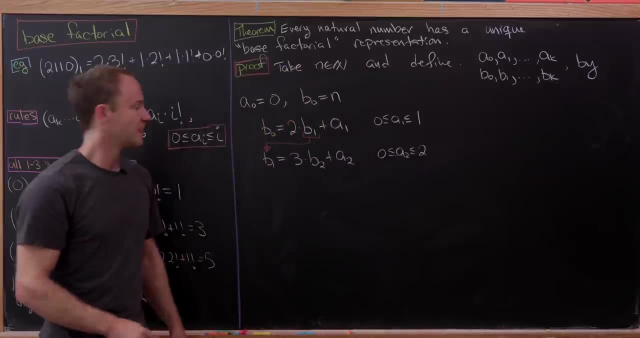 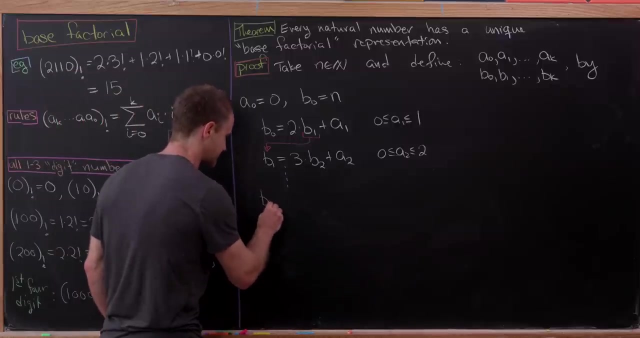 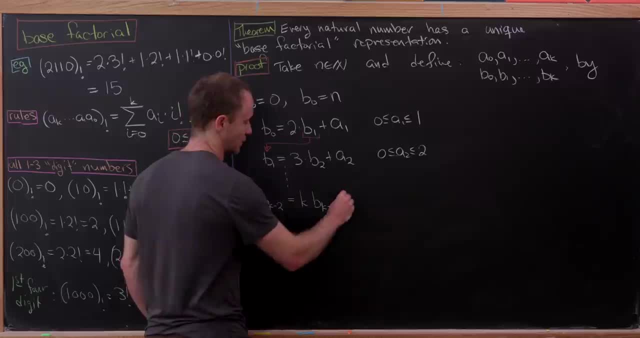 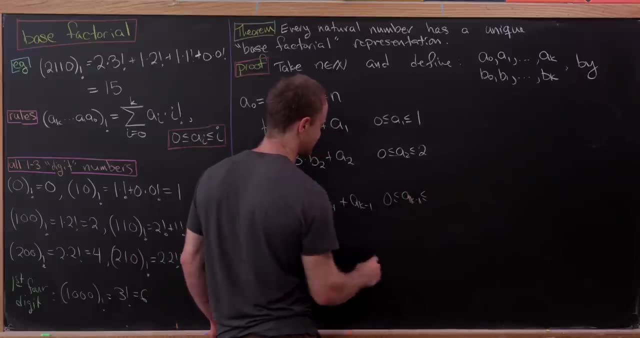 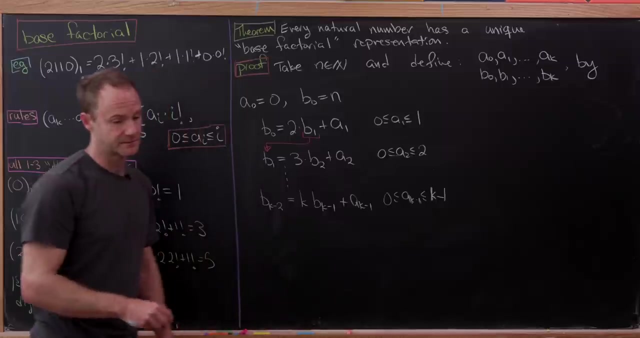 k times: bk-1 plus ak-1, and here ak-1 goes between 0 and and k, and here ak-1 goes between 0 and and k, and here ak-1 goes between 0 and and k minus 1. okay, great, and then we'll go one more time, so we'll have this BK minus 1. 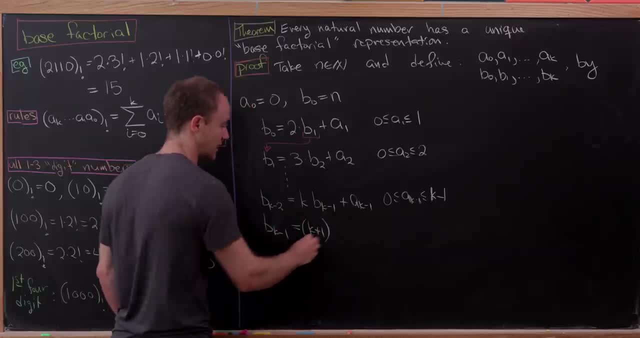 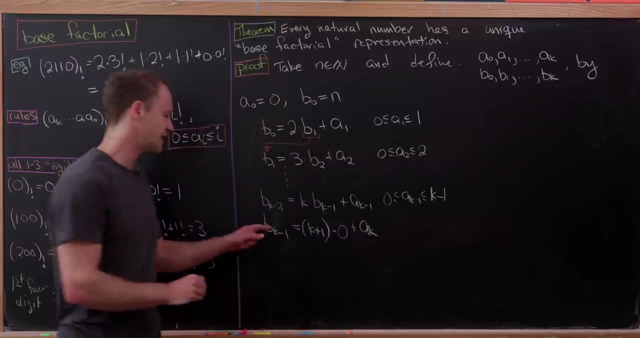 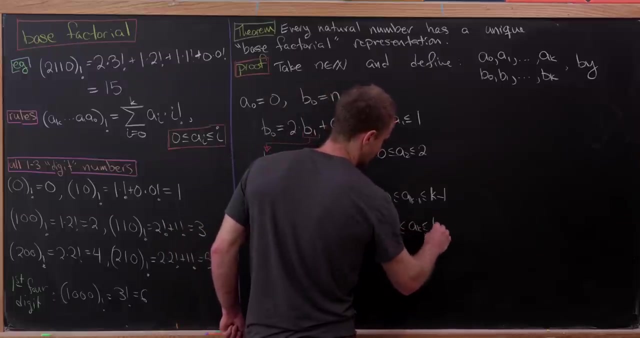 and we're gonna divide it by K plus 1 and we'll get a quotient of 0 and then our final remainder, which is a K, which I guess we could see. that BK minus 1 is a K in this case, and a K will be between 0 and K. and now all we have to do is prove. 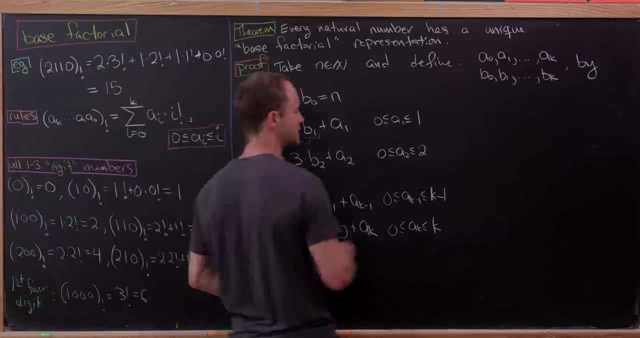 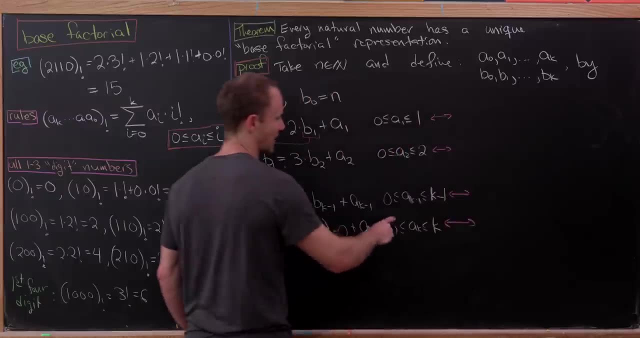 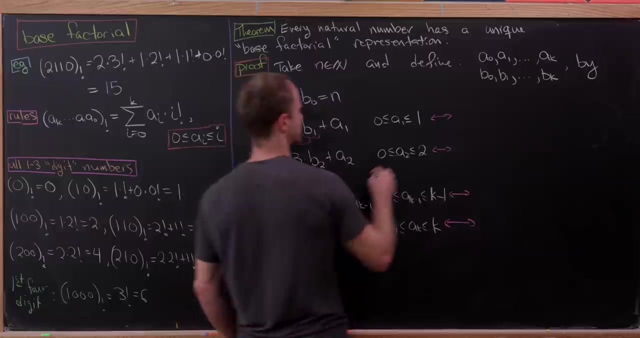 that we have indeed built the representation. but before we do that, I'm going to take these equations and invert them a little bit, and you know, I know that I'm putting the arrow next to the size of the remainder, but it should be really coming from over here, okay, so notice that we can write a. 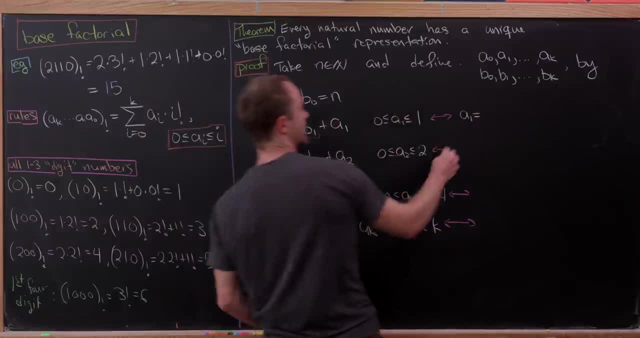 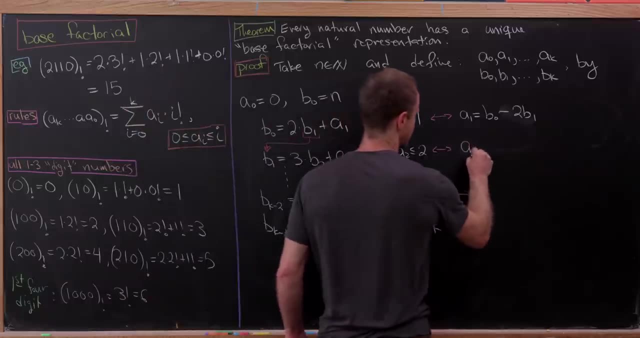 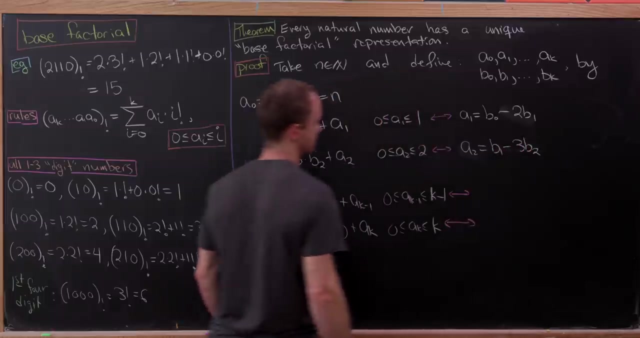 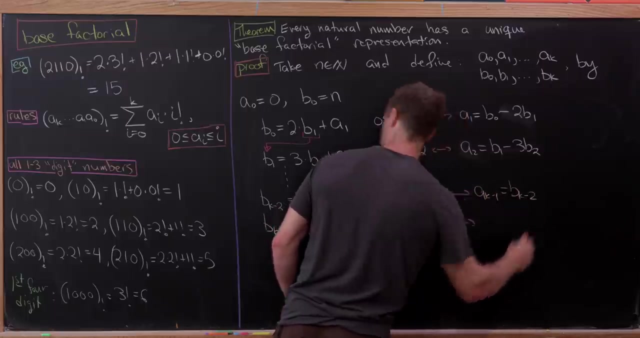 A1 is equal to. let's see B zero minus two times B one, and then we can write a two similarity, Goodness. So a2 will be: let's see b1 minus 3b2.. Then let's see ak minus 1, which is occurring way down here- will be bk minus 2,. 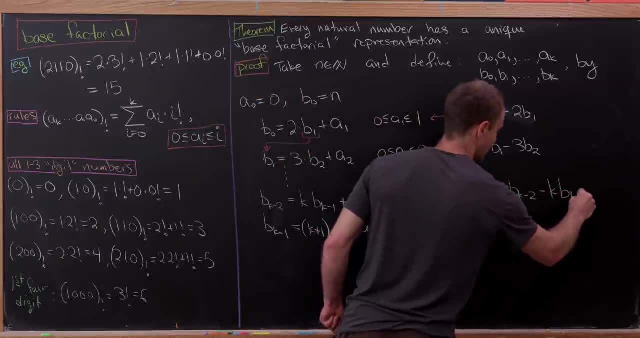 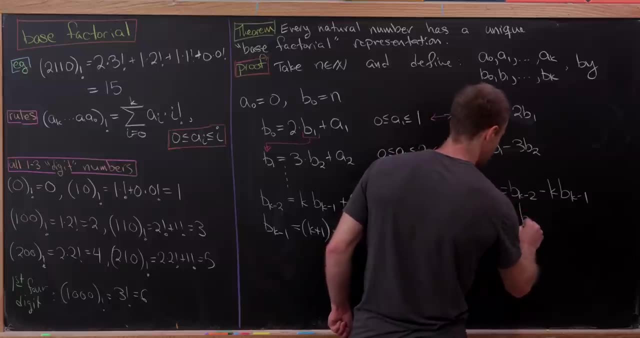 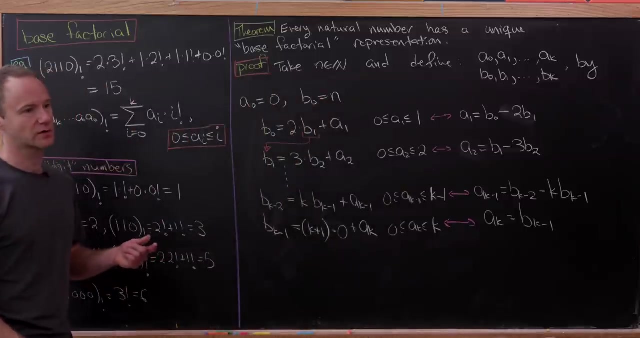 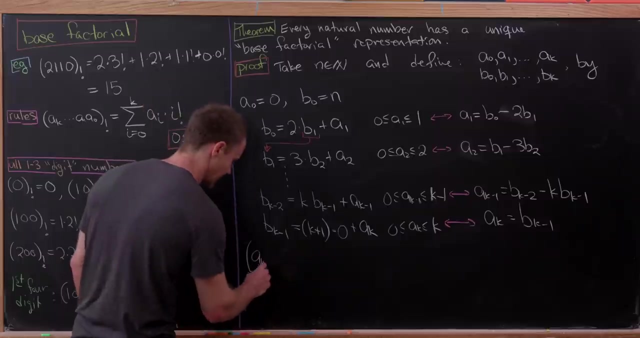 and then minus k times bk minus 1, and then finally, ak will be bk minus 1.. Okay, so that's good, And now let's look at the base factorial number with those digits that we've just created. So we start here at ak. the next one is ak minus 1,, all the way down to a2, a1, a0.. 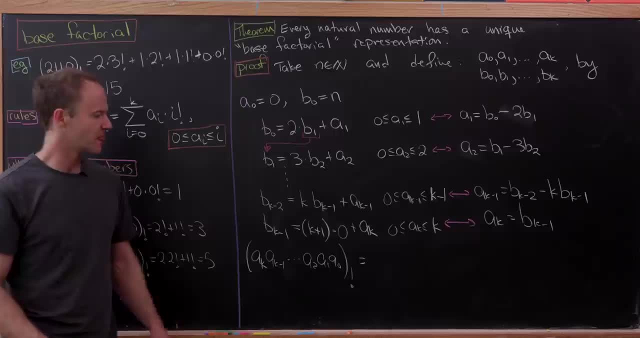 And, like I said, this is like base factorial. But instead of writing these as like, for instance, ak times k factorial, ak minus 1 times k minus 1 factorial, I'll write this. I'll write them using the expression that we've created by inverting these defining equations. 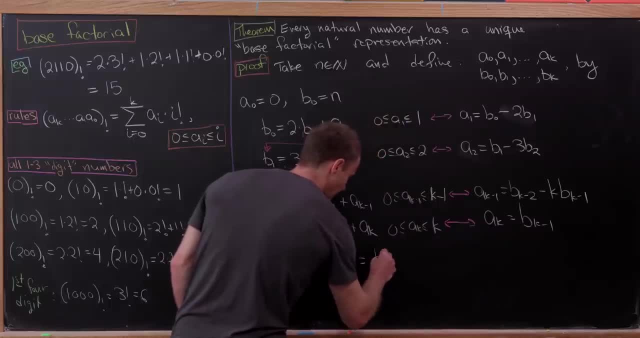 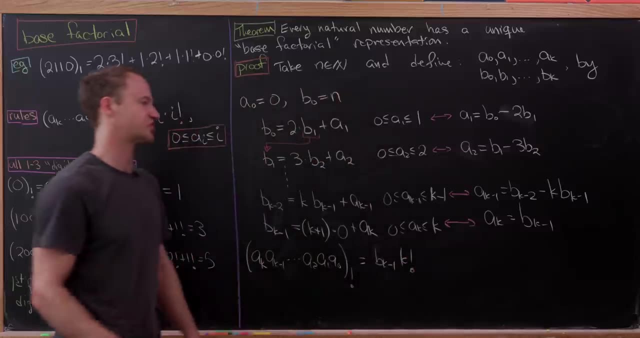 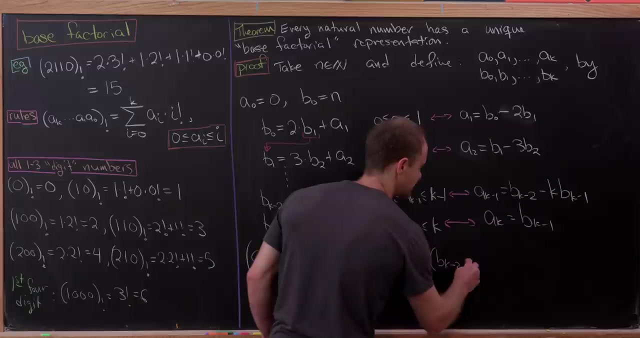 So that's going to start with this over here. So we'll have bk minus 1 times k factorial. That'll be like our first term. Oh, and then what comes after that? Well, it will be bk minus 2 minus k times bk minus 1 times k minus 1 factorial. 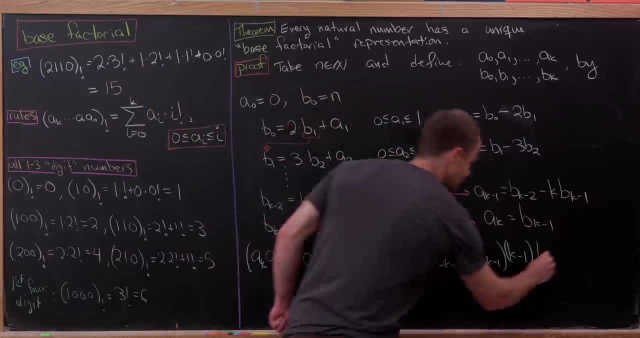 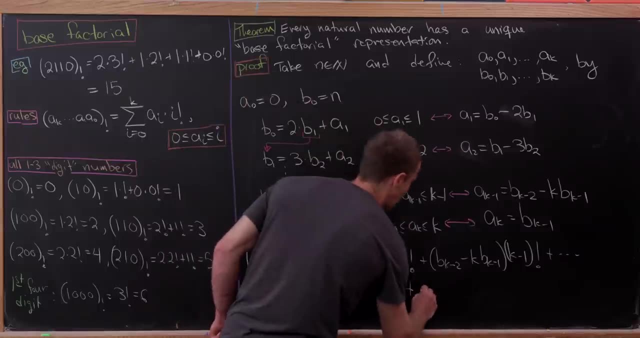 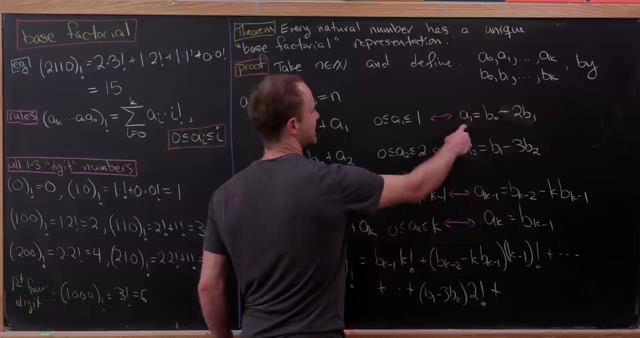 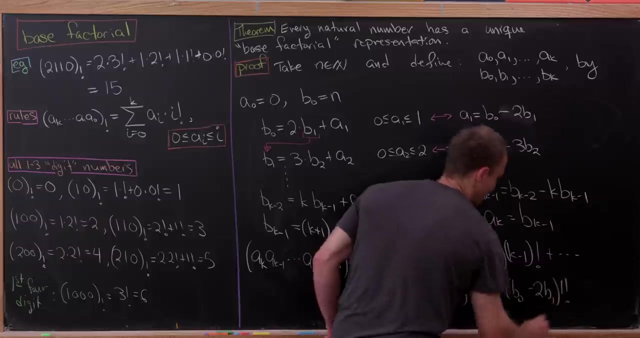 From this next one, And then that's going to continue on, and on and on, And then let's see Down here, we'll have b1 minus 3 b2 times 2 factorial. And then finally this term right here, which is b0 minus 2 b1 times 1 factorial. 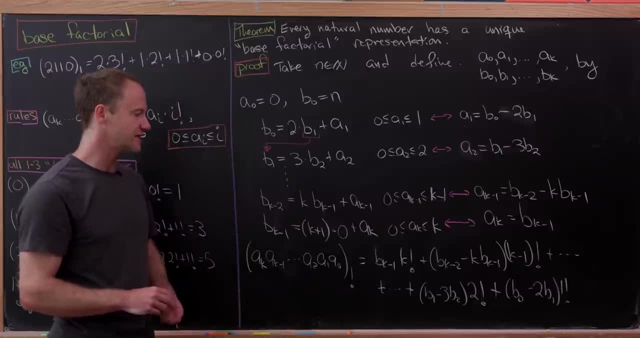 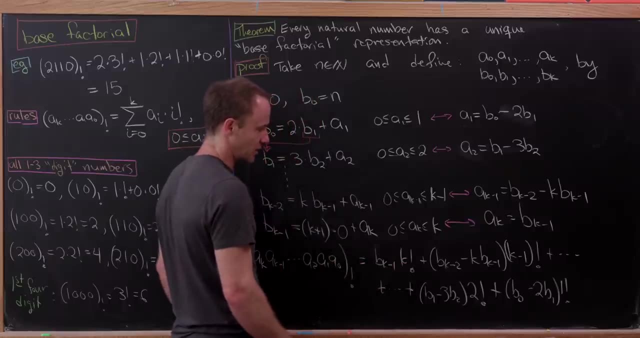 But I think like, if you're sharp-eyed, you've probably already seen this. You've probably already seen this. You've probably already seen what is going to happen. Everything is going to collapse. So look at this: bk minus 1 times k factorial will get canceled because here we have bk minus 1 times k times. 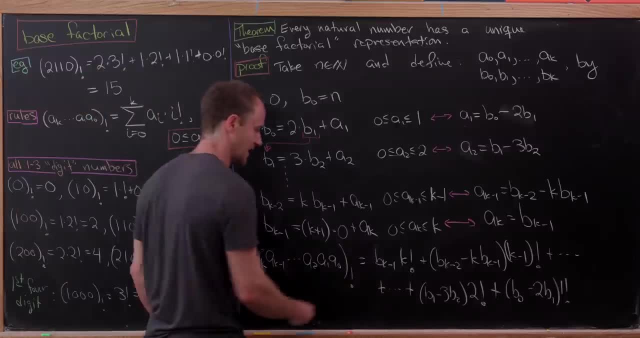 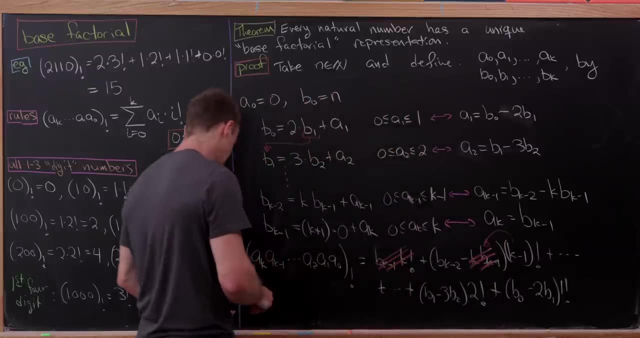 k minus 1 factorial, and it's attached to a minus sign, So we can see that this object will be canceled with this well, after it's been distributed through. And then this kind of thing is going to like continue on, and on, and on. 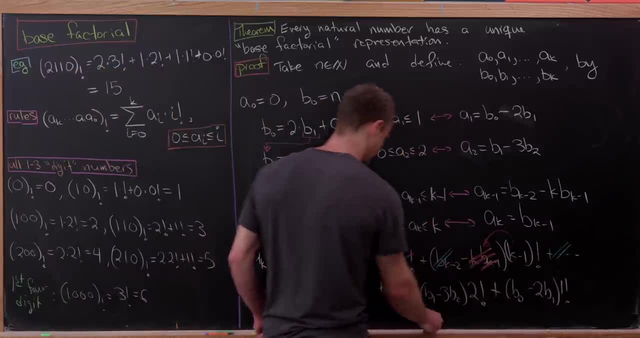 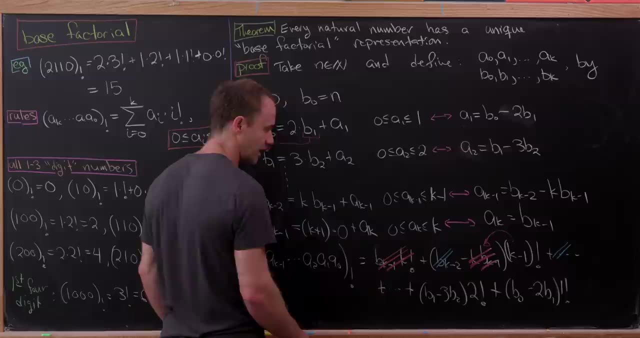 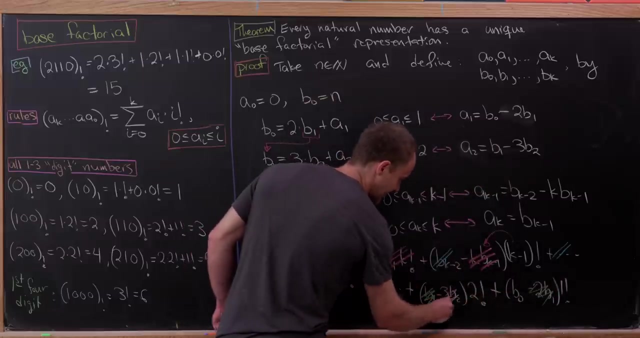 So this bk minus 2 term will cancel with something that is coming Afterwards. then let's see what's happening at the bottom. here We have minus 2 b1. Oh, and here we have 2 b1. So this b1 will cancel with this b1, and likewise this 3 b2 times 2 factorial. 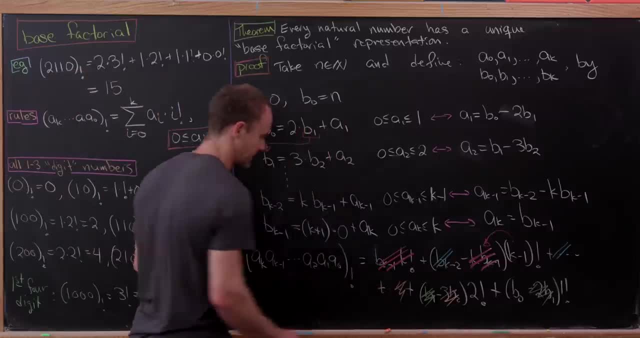 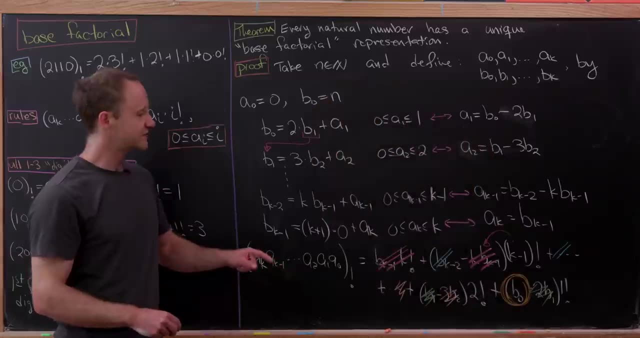 which is really 3 factorial times. b2 will cancel with something that comes before. So what's the only term left? We'll notice that it's this b0 term, but we started by defining b0 to be n, So this is in fact. 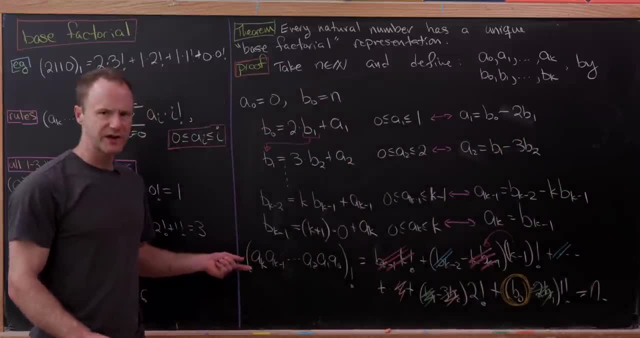 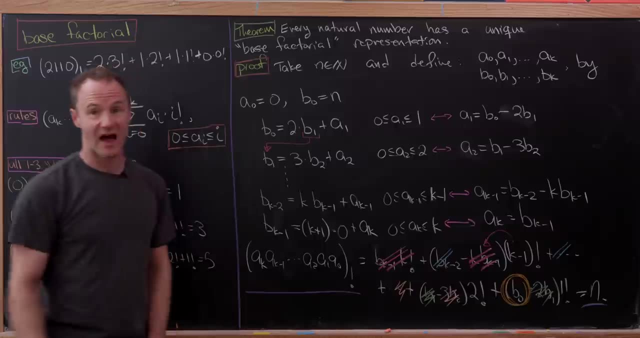 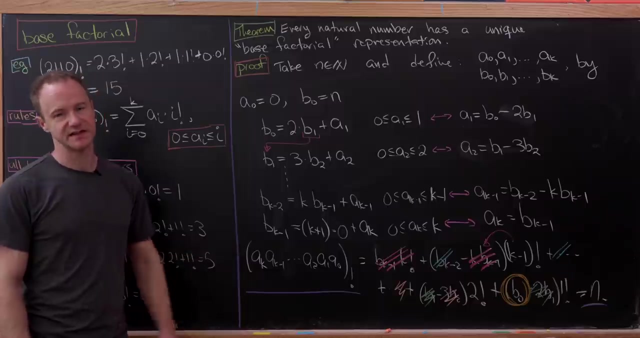 equal to n, which means: well, what have we done? Looking at the extreme left and right hand side of this equation that we've built, we have a factorial number system representation of n. So that proves that there is a representation. Now let's finish it off by proving that it's unique. 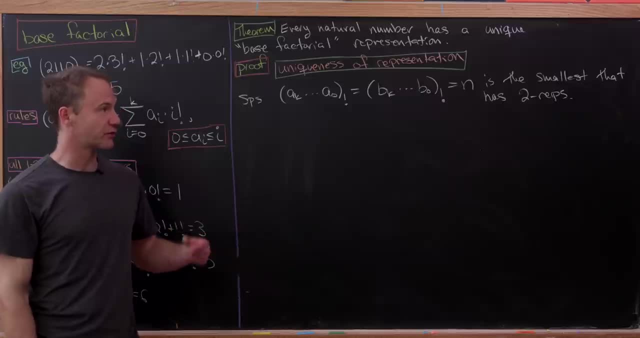 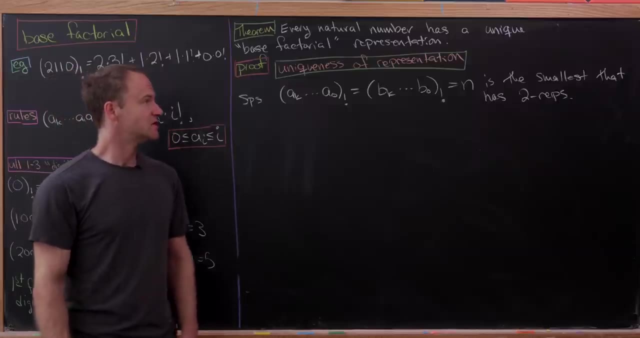 We've got one last thing to do, and that is to prove that we in fact have a uniqueness of representation into this factorial number system. So let's suppose we've got a number n, which is the smallest natural number that has well. 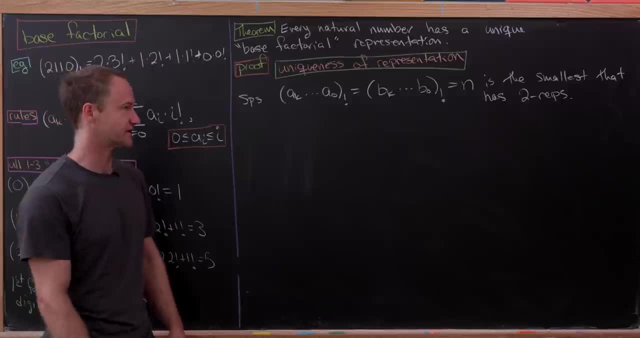 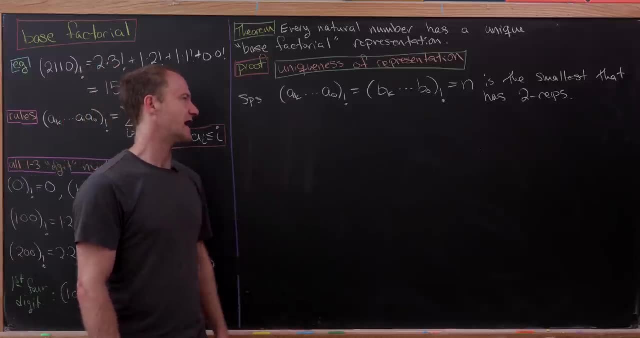 at least two representations in this factorial number system And here I've written them and I'm reusing our a sequence and our b sequence. So we've got ak down to a0- sub factorial and bk down to b0- sub factorial And I guess there's a little argument that you need to prove that these have the same number of digits. 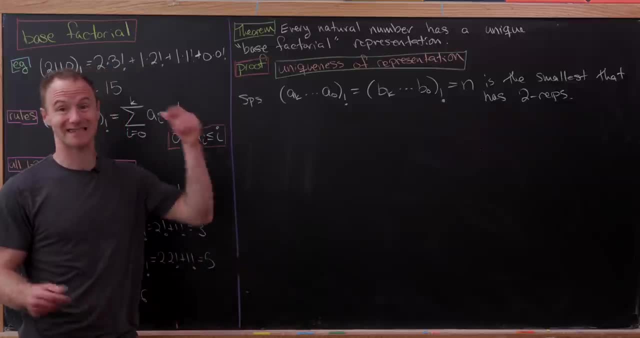 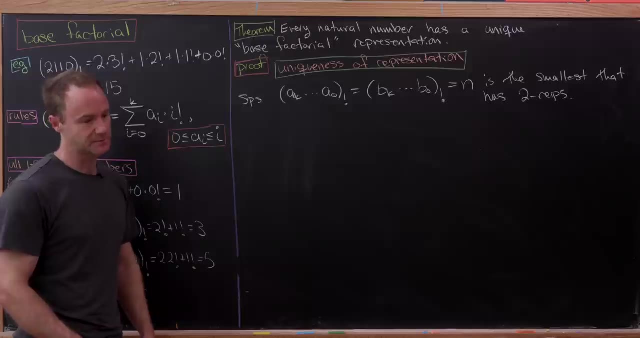 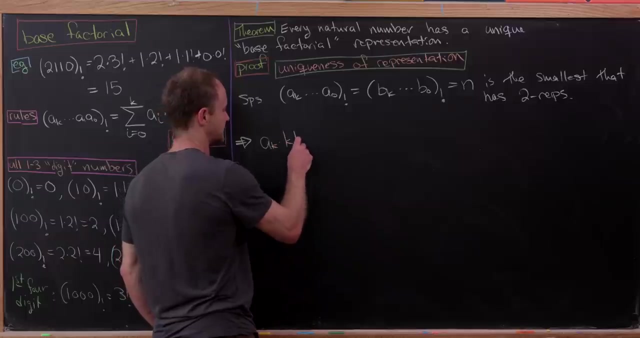 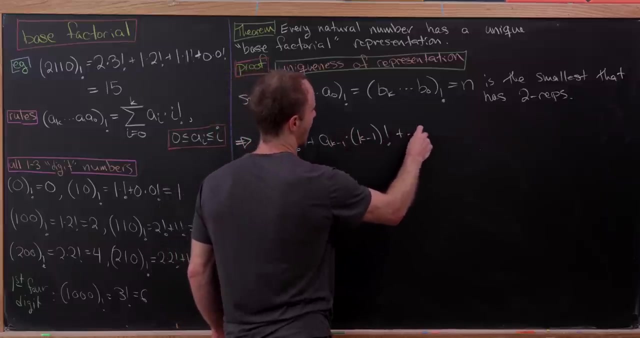 But I think this thing we started out we've with the size versus the number of digits is good enough to say that these have to have the same number of digits. Okay, so now let's write this out. So this means that we have ak times K- factorial plus ak minus wanna times K minus one factorial, added all the way down to: 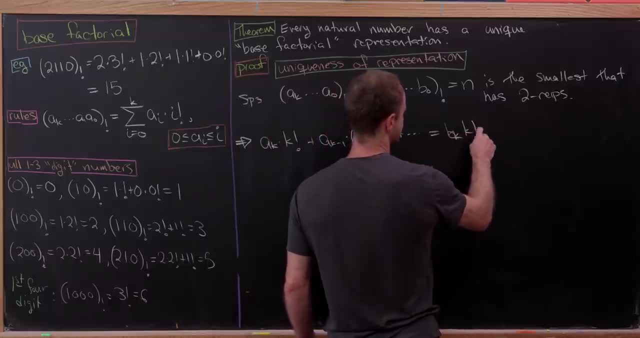 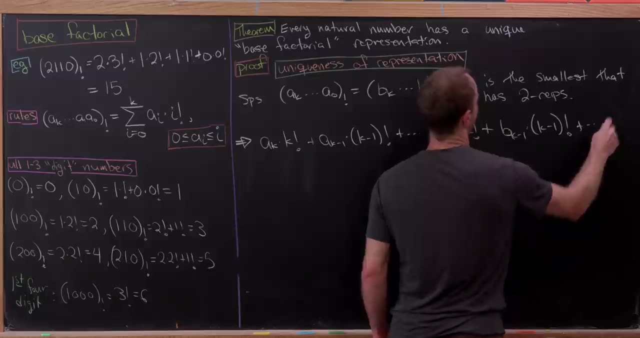 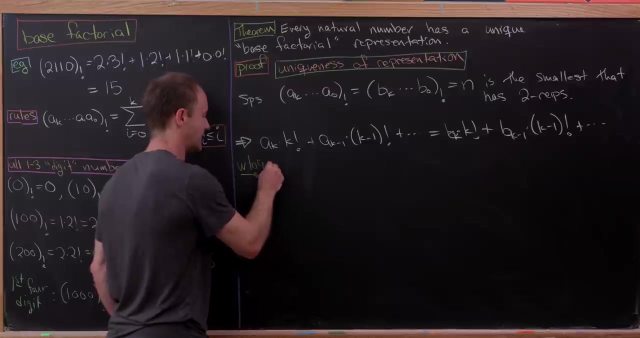 the ending point is equal to bk times K factorial plus B. k minus 1 times k minus 1 factorial, plus all the way down. And now let's notice that by the minimality of n, we know that the first digit of each of these is not the same. So in other words, 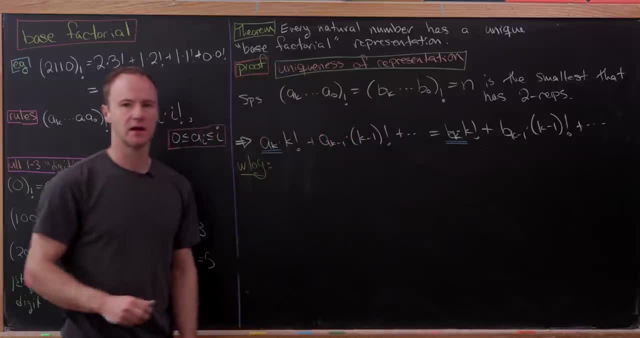 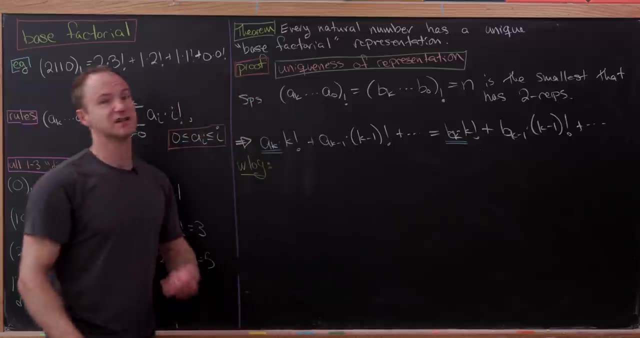 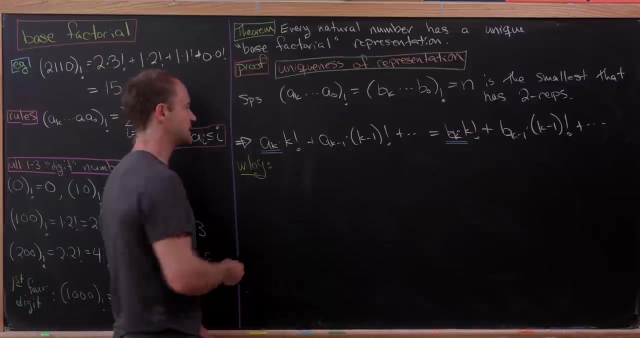 the ak cannot be equal to the bk. And well, why is that? Well, that's because if they were equal, we could just cancel them off, and then we would have a smaller natural number that did not have uniqueness, But we've assumed that we've got the smallest one. So let's, without loss of generality. 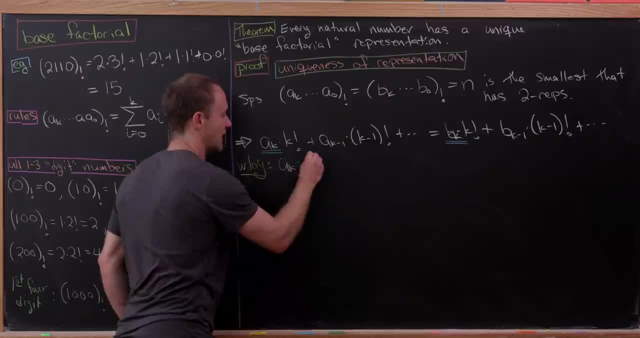 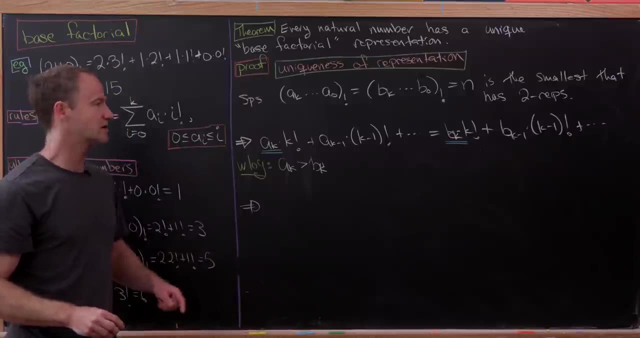 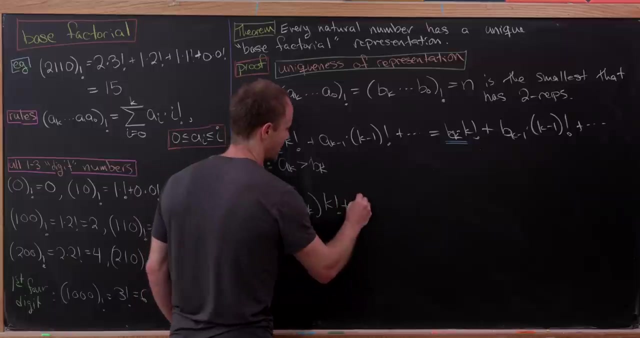 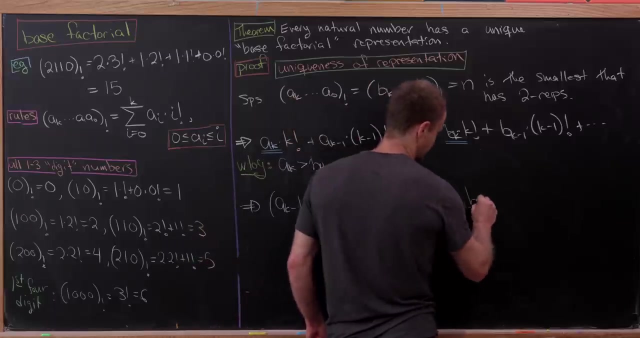 assume that ak is strictly bigger than bk, But that sets up a problematic equation. And what is that problematic equation? Well, let's write it down. So we'll have ak minus bk times k factorial plus ak minus 1 times k minus 1 factorial. all the way down equals bk minus 1 times k minus 1 factorial. 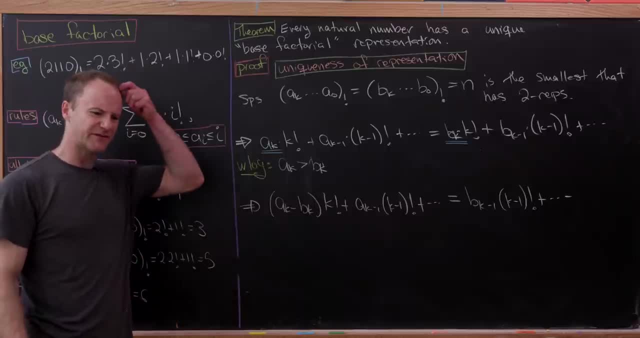 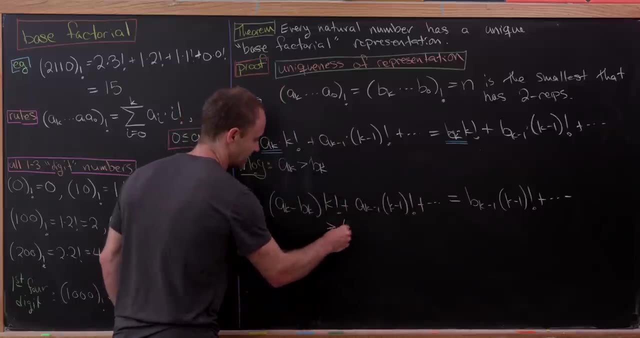 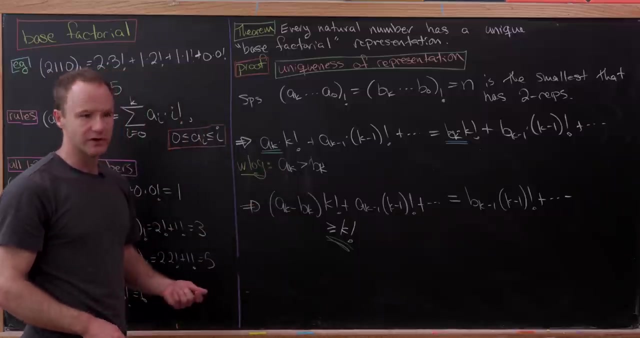 all the way down. But look, these have different numbers of digits And that's the problem here. Notice that this left hand side is most definitely bigger than or equal to, k, factorial, And we know that's true because ak is bigger than bk, which means they're different. 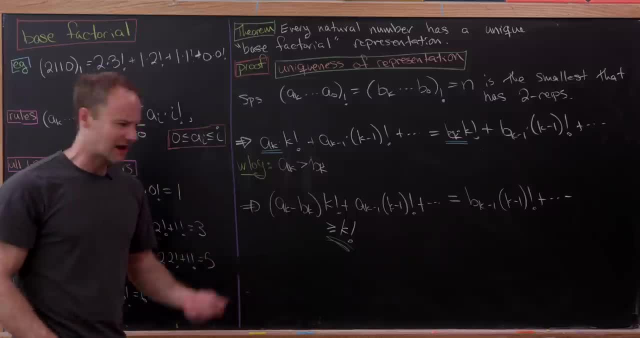 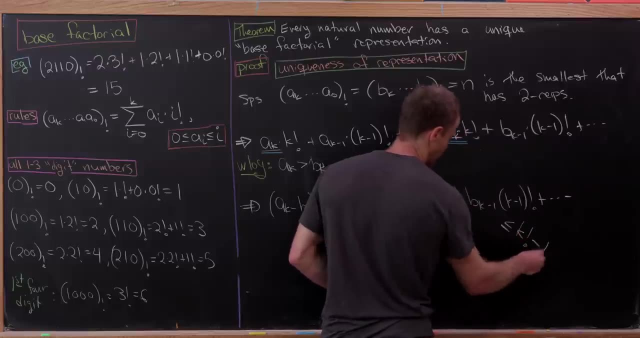 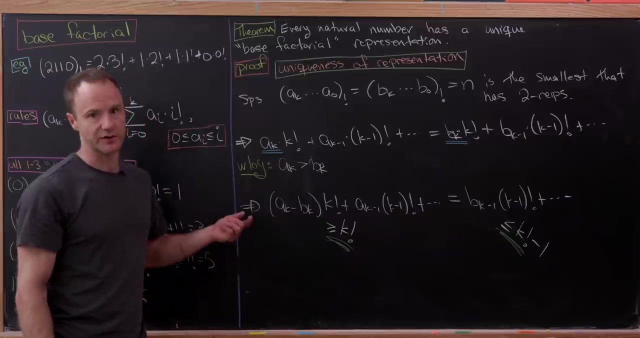 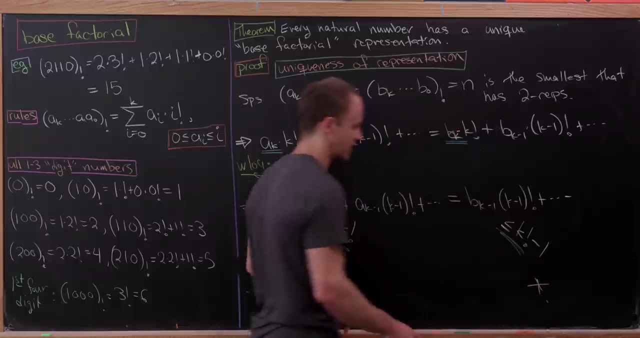 And we know that this right hand side is less than or equal to k factorial minus 1.. But you can't have a number that's simultaneously bigger than or equal to k factorial and less than or equal to k factorial minus 1.. And that is where we get our contradiction, Contradicting the idea that it was. 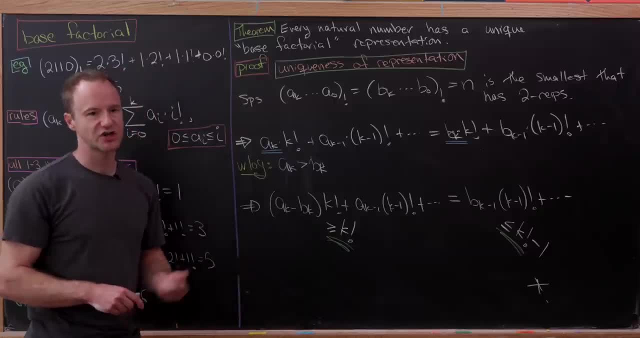 possible to have a number that was bigger than or equal to k factorial, And that's where we get our contradiction. But we also have a type of non uniquehan multiplier, which is a super important representation in this factorial number system. So, if you're still around, thanks for sticking around so long, And if you haven't subscribed yet, 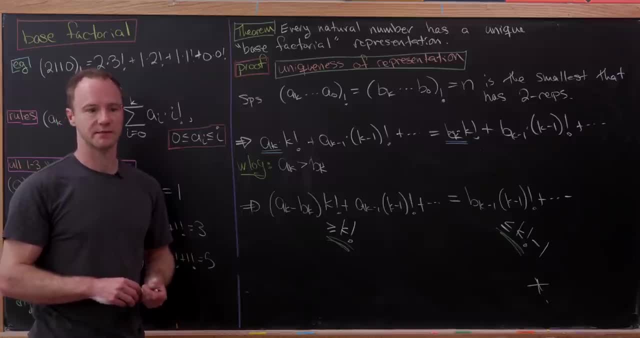 maybe consider subscribing. It would really help us out, And that's a good place to stop.